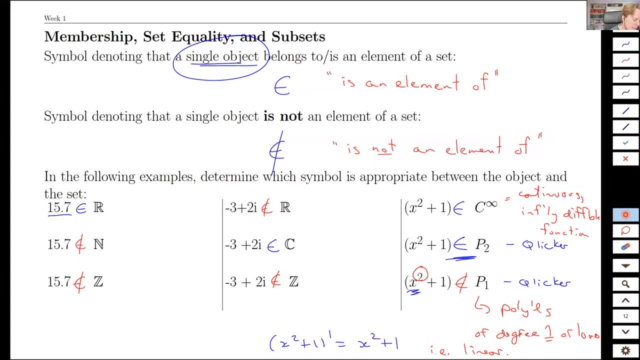 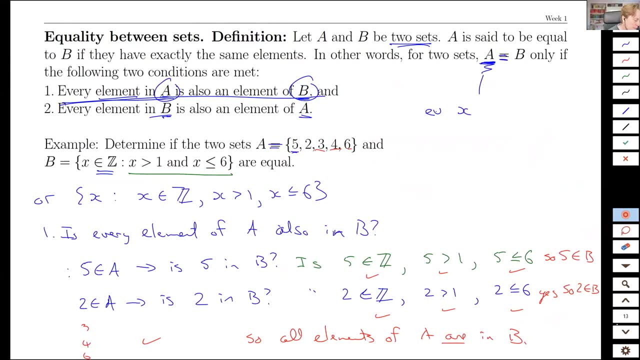 That gave us something useful for individual elements. But of course if I had a bunch of different numbers I could ask: are they all in the reals or not? That kind of question. And the notation we use for that is subset notation. 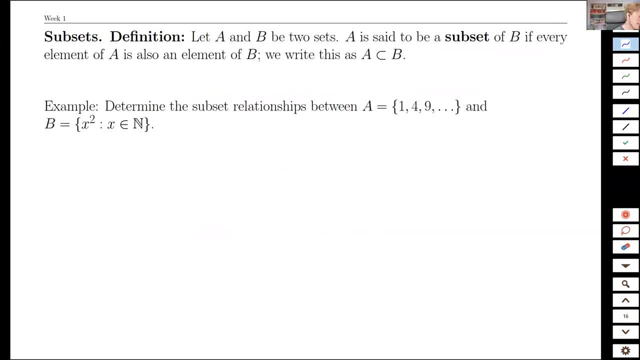 And it's done by the sort of curly or smoothed out sideways U. So this is the subset operator indicator And basically this is easier to see with a Venn diagram. So if you have a set A and you imagine it's represented by some circle here, if you've never seen a Venn diagram, let me know. 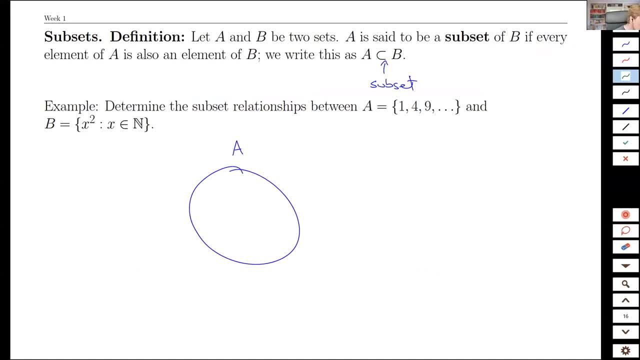 I imagine this is even through popular culture. it's been something we've all seen. So if we have A and another set B inside of it, then we would say that B is a subset of A. Now, more formally, we could take a look at these things here. 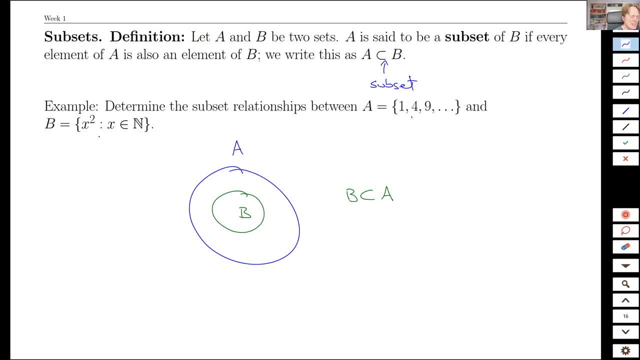 In the interest of time, I'm not going to go through these particular examples. They're not the kinds of things you see in your homework anyway, So I think we're going to spend our time moving forward to the future notes. But this intuitive idea of something being a subset of another is. I think most people don't struggle with this concept. 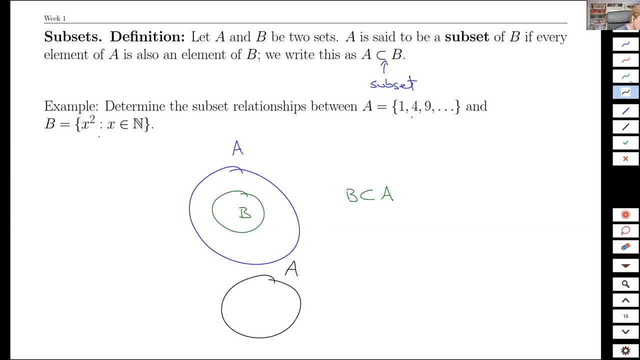 So I don't want to spend too much time. If you had A here and then B had some intersection but was not completely inside of A, then what we would say is that, while B here is not a subset of A and, furthermore, A is not a subset of B, 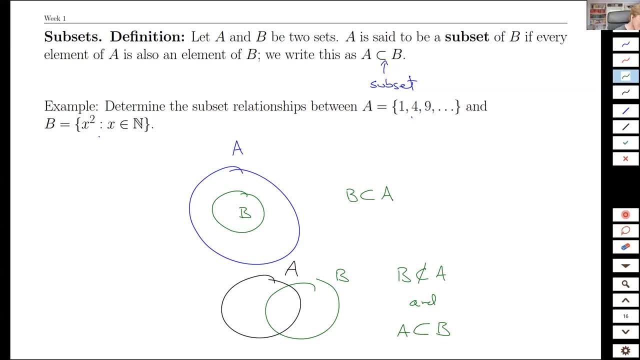 So it's easy to have these turn into Cs and try to make them explicitly look like a subset, sideways U. Now the border case is actually interesting And that's where we have the same set. So if we have A and B is actually all the same values, all the same letters, all the same numbers, whatever we're defining our sets as. 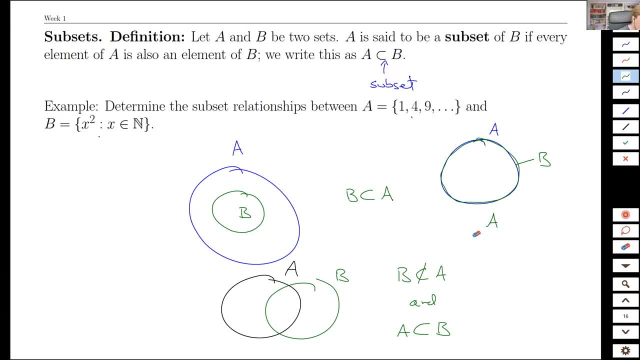 then we would have this interesting relationship that B is a subset of A. We would say that And we would say that A is also a subset of B. Some of you may have seen a version of the subset thing where we add an extra bar here. 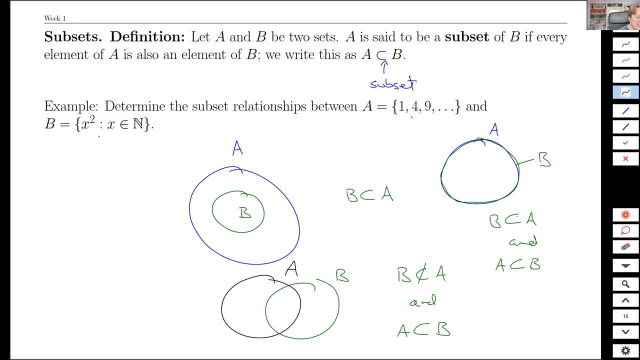 We don't do that Here. this in this subset can be is like: less than or equal to, is factored in here. If B is contained in A or is equal to A, then that will still use the same symbol for all of those. 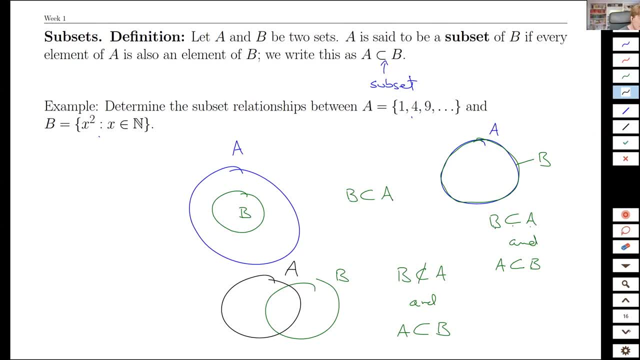 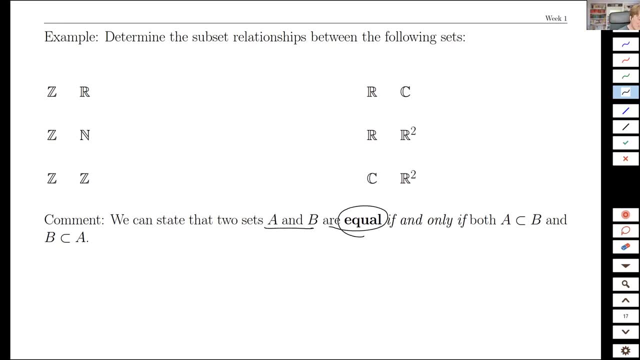 And the reason that is it makes some of the other things you want to do next a lot simpler. Specifically, if we have two sets that are actually equal- for example I just drew for you- then they are equal if, and only if, we can say that A is. 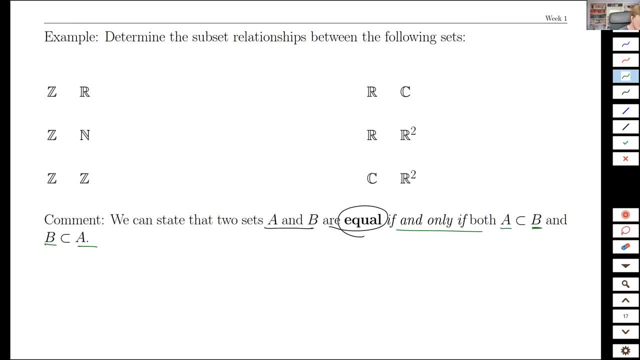 always contained in B and B is always contained in A. So that's another equivalency that we can say. A is equal to B is the same as A is all contained in B and B is all contained in A. trying to make these look as typeset as possible. 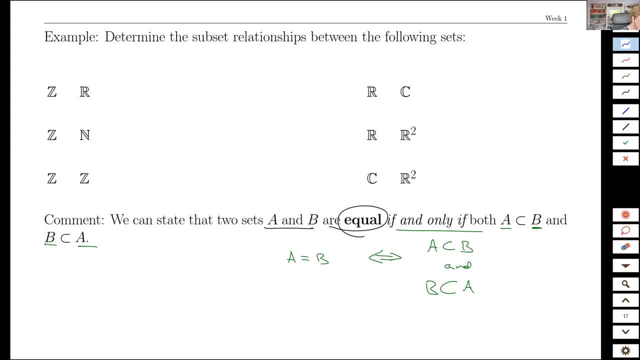 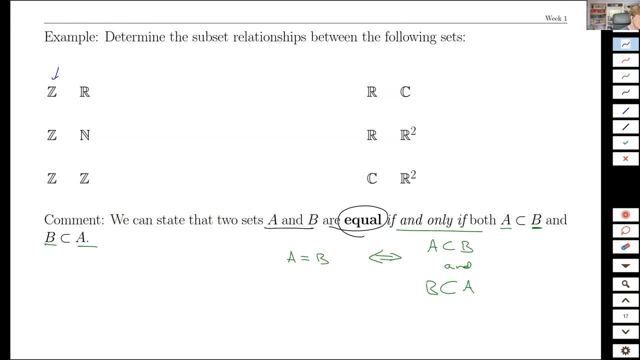 There's a lot of stuff going on here. There's a lot of stuff going on here Because it's a good reminder of the definition of what these Zs here, Zs are the integers, And those are again including negative numbers. 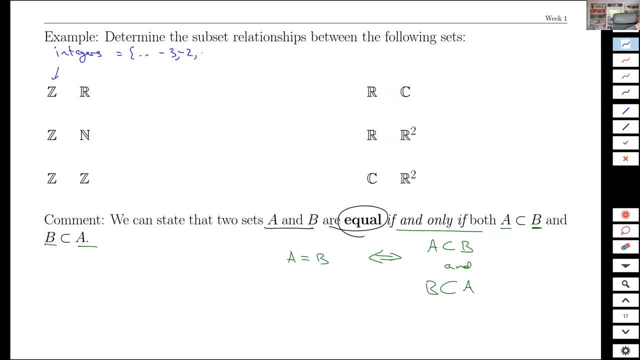 Oops Minus two would usually be in that set, in that order, And one, two and so on, And so we would say that is a subset of the reals. Why? Because every element I can list here that's in the integers is a real number. 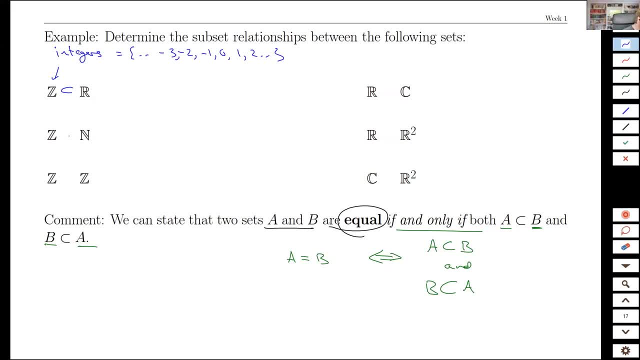 So we can use that. We would not have a subset operation this way, because what's N? N is what we're calling the natural numbers, And for the purposes of this course, the natural numbers includes the number zero and then all the positive integers. 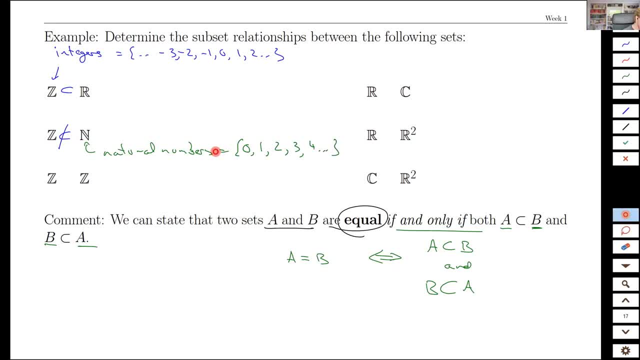 And it's very clear that a number like minus three is not in this set, so we cannot have Z being a subset of N. However, we do get these kinds of trivial subset things like: is the set of all integers the subset of all integers? 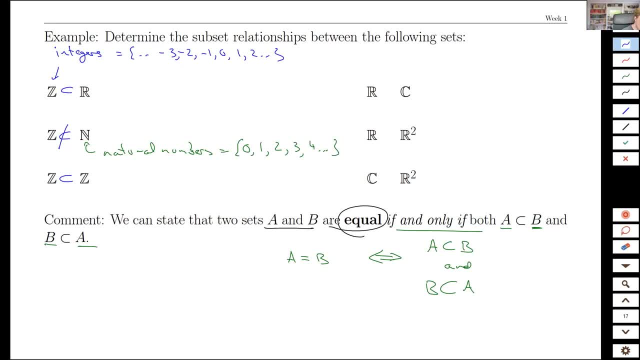 Well, yes, sure, because they're the same thing And we're going to this kind of relationship here where if two sets are equal, then one is always a subset of the other. The other ones are. pretty much what you'd expect. 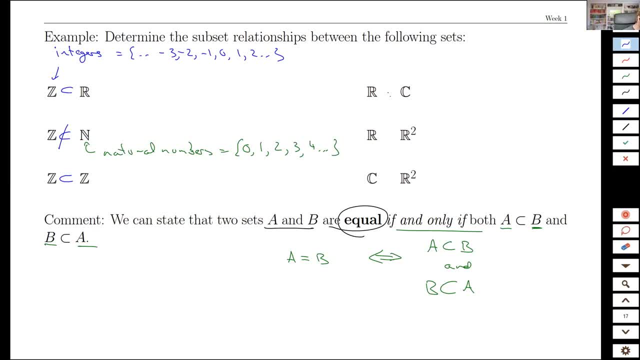 Maybe not entirely actually. So the reals and the complexes, For these we'd actually probably say no to all, All of them, Unless we added some extra caveats, some extra space things. In particular, this one's probably the toughest one, and we can get into debates about that. 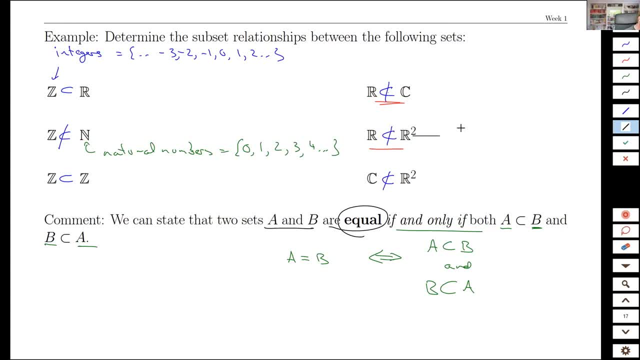 These other ones are more clear. You might be thinking of R2 as the plane and then you think of the real line as one set of real numbers. That's true, except the way we represent these things is that the R-squared values points on a plane are defined by a tuple. 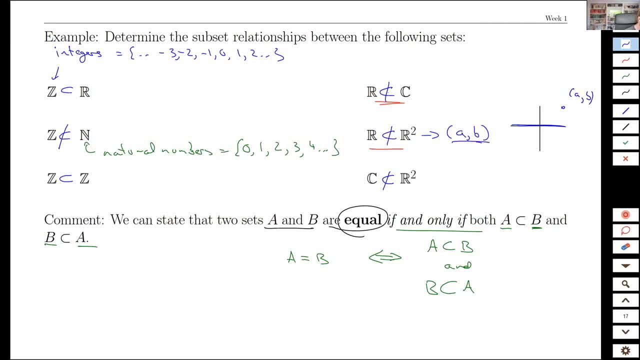 So it's a, It's a combination of two values, two real values, whereas this is just a single value, c, And so these are sort of incompatible forms. There is a relationship between them, incompatible, But we can't say that the number c is somehow in the set of pairs of numbers, pairs of real numbers. 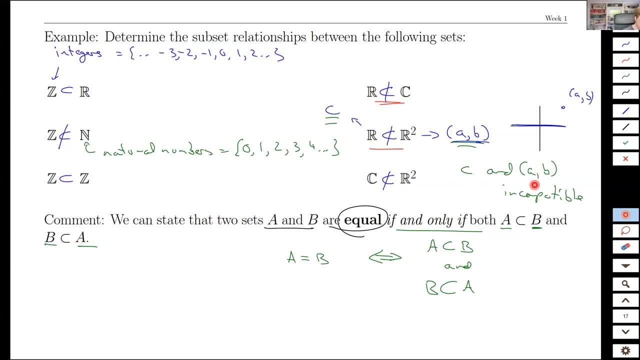 That just doesn't make any sense. They're not the same data type, if you like, if you're a computer programming person, The same thing for the complexes and the reals. Like we draw this as a plane, we draw this as a plane. 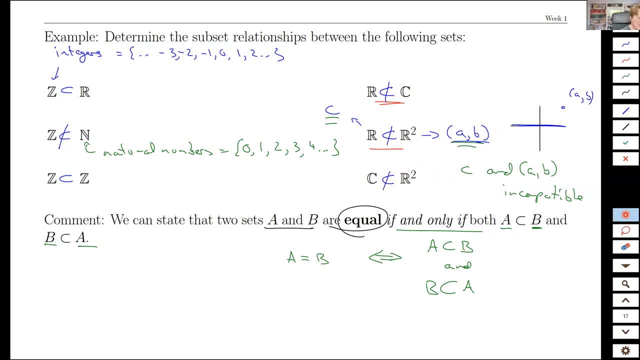 There's some parallels, but they're not subsets of one another, So we have to. This points to the possibility of other kinds of relationships besides subsetting. that could be useful. And sorry, going back to here, Absolutely, If you went to this order, you would have that the natural numbers are a subset of the integers. 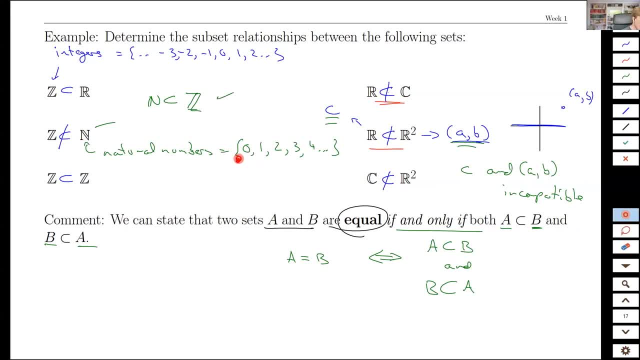 That would be absolutely true, Because 0,, 1,, 2,, 3,, 4 is contained in the set of integers as well, And there's some leftovers. but that's fine. This is a smaller set and every element in the smaller set is in the larger set, so that would be perfect. 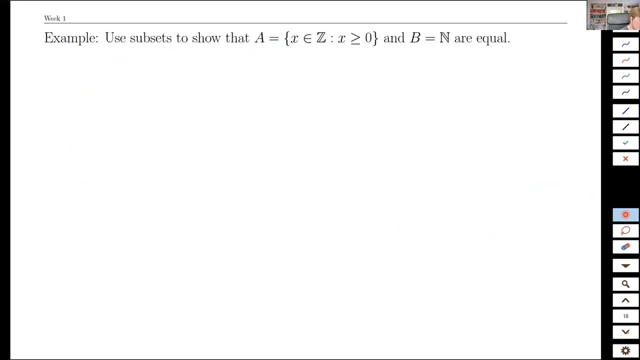 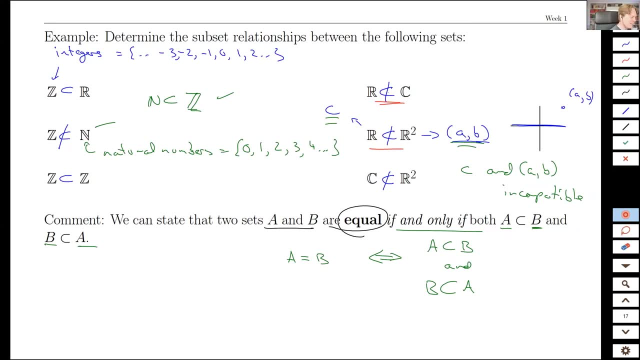 All right, I think we're going to stop there for the week. two notes, or sorry, lecture, two notes. Yeah, these things tend to be kind of tedious in terms of the proof that one thing is a subset of the other And it's not a central focus of the course. 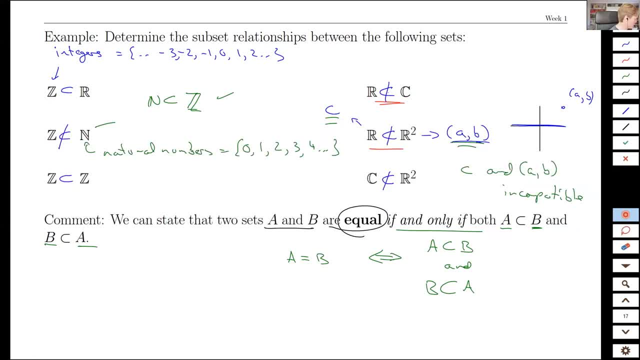 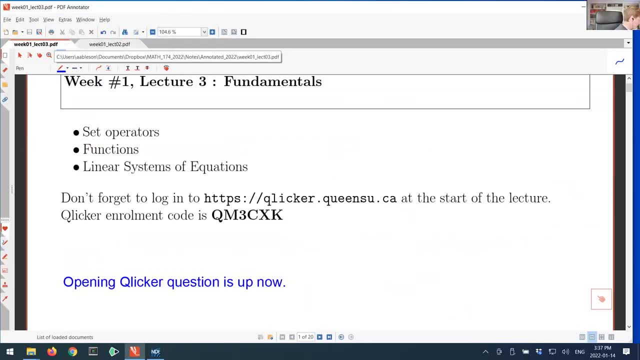 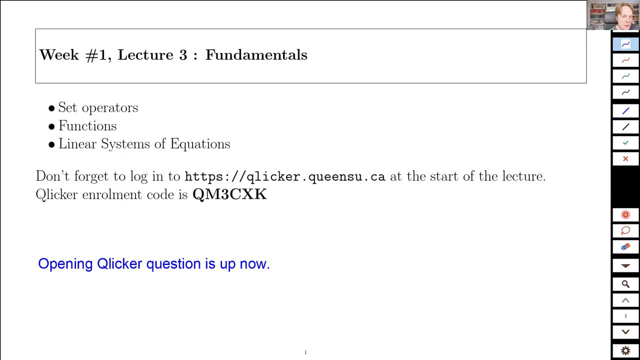 This is just getting us some concepts that we can use, So let me just save that always good policy Control-S, and then we'll move on to today's notes. All righty, So I'm sorry for anyone who hasn't already logged on to Clicker. we'll have a couple of questions scattered throughout the lecture today. 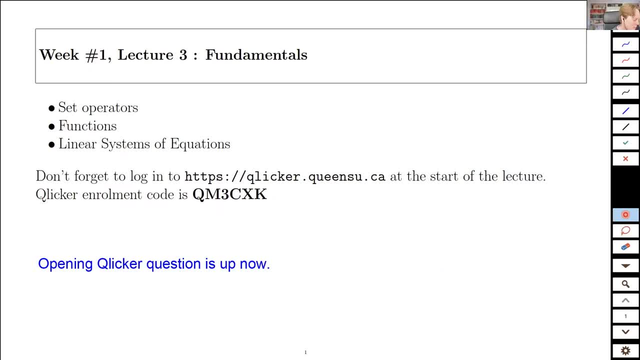 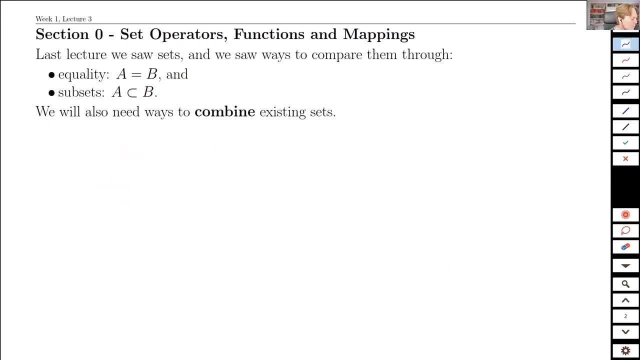 And the access code again if you need it is that QM3CXQ rolls right off the tongue, All right, so We've seen these two operations now very recently, and there's obviously other ways we can combine sets. 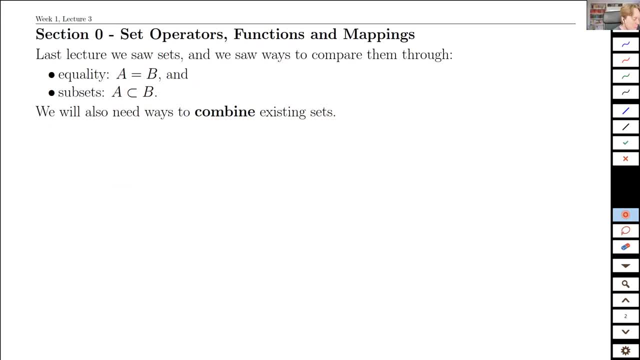 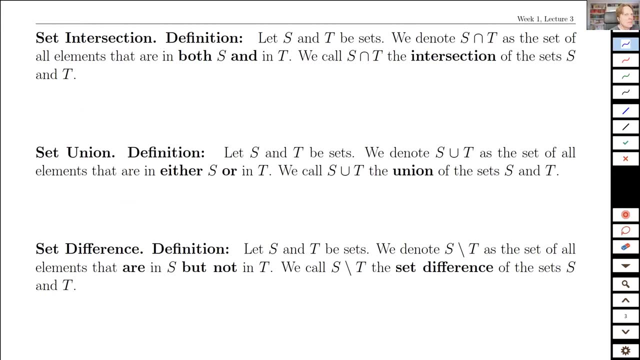 So this is comparing sets, but we might have sets that we want to put together. take apart that kind of thing, And most of you will again stop me if My impression is that most of you will have seen these operations, whether you formalize them or not, but you've seen them before. 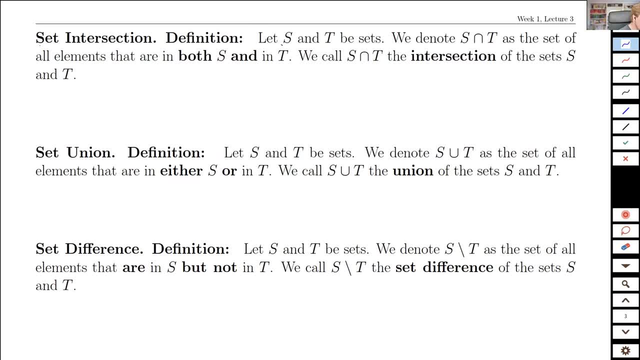 The idea of a set intersection. So let's start off with two sets. We're going to call them S and T For the purposes of this page and what I think of this, as it's like an N shape, And so it's easy to remember that N shapes are intersections. 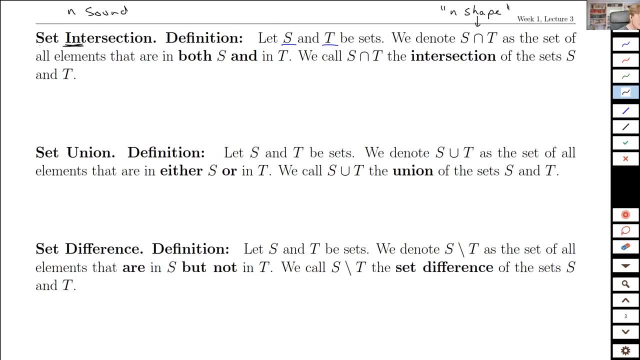 So an N sound. So that's the reminder that this is the intersection symbol, And Venn diagrams are going to come back to our assistance here as well, If we had the two sets, S and T, and the idea is that we have individual elements in here. 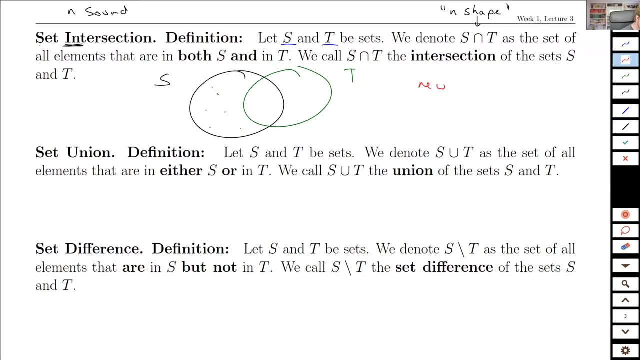 then We're going to get a new set. The new set, S intersects with T, is equal to this region here, Which is equal to all elements- let's call them X- that are in A, S and that are in, or elements of T. 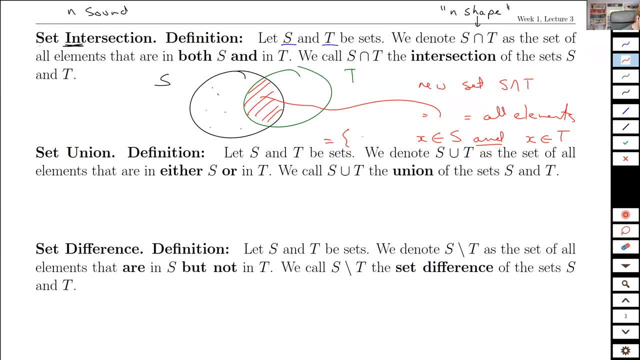 And so we can actually formalize that a bit better. It would be a set of X's, such that X is in S and X is in T, And not a huge shocker for the next one. For the union, this has sort of a U shape. 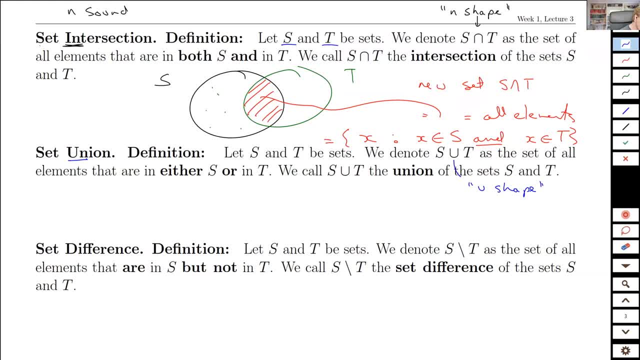 So that's your mnemonic for remembering. that's the union symbol. Then for this we have the same kind of Venn diagram. We might have two sets, And the union is going to be anything that isn't either one of them. So this is like adding: 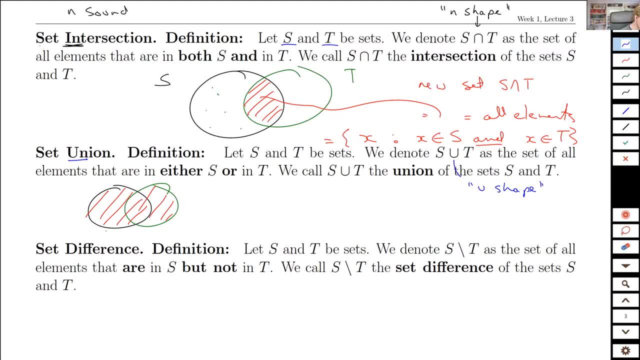 This is not quite like subtraction- We'll talk about subtraction in a second- But this is like pooling the two sets together, And S union T would be a set of elements such that the element is either in S or it's in T. If I can take all the elements of S, they're going to be in the union. 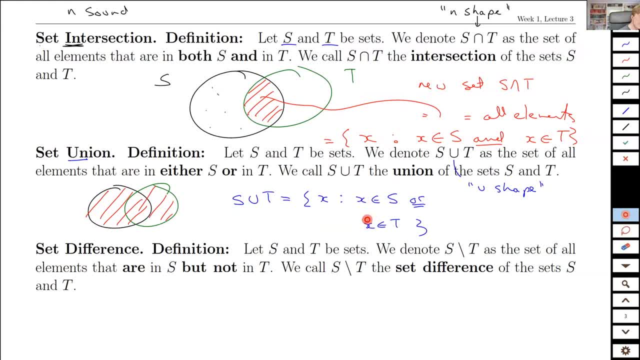 And I take all the elements of T. they're going to be in the union, And if there's any overlap that's okay, Because sets just ignore duplicate values And so we would get this collection here. Let me draw the borderline. 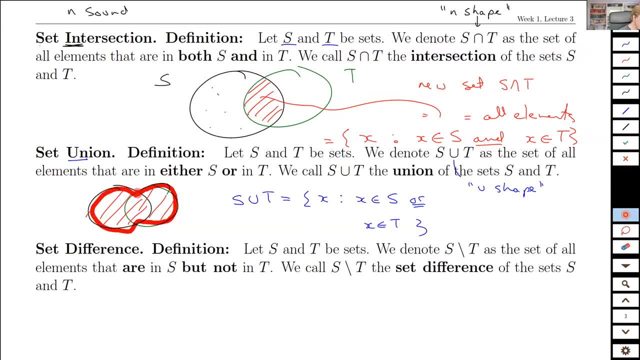 This entire set. here is what we would graphically need to notice as union T. Now, last but not least, in the notes in the online textbook we have the set difference. I was just speaking with the other instructors today And looking forward. this one actually doesn't get used very much. 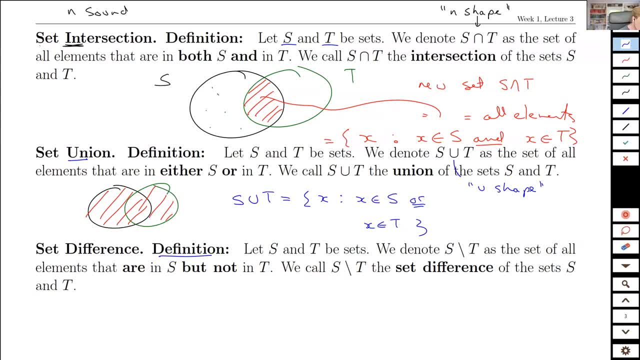 So this one feels a little weird, Then that's totally fine. Basically, you can think of this as a set S minus T. Again, it's not minus, but we're going to take out all of the elements from T that are in S. 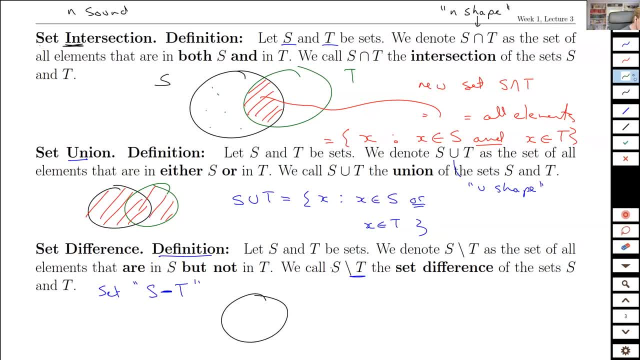 And so if we did a Venn diagram for that And give it some labels so we know which one's which. Sorry, I should have done that here before as well. S and T. So we have all the elements in S And we're going to keep this set difference. 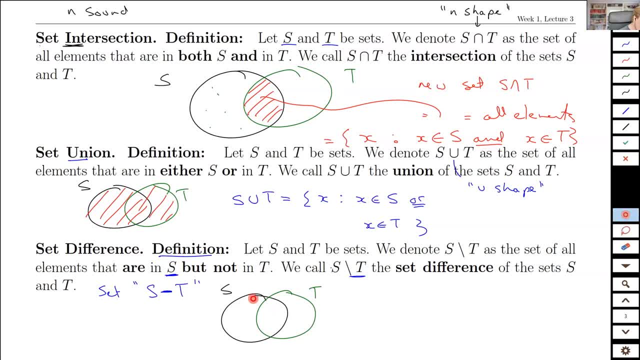 The things that are in S. So we're starting with this pool here, We're starting with this, And then we're going to subtract the things that are in T. We don't want anything in T, So we're going to keep anything in S that's not in T. 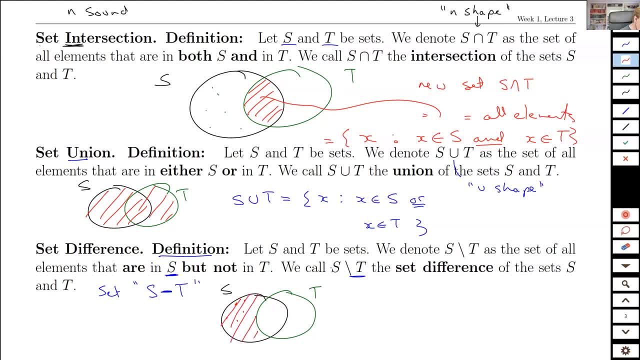 That's these guys, these guys, these guys. One fact: that's everything up to the overlap. So it's this shape here. that would be our set S intersection: T, Sorry S difference T. So notice it's sort of like the opposite of the intersection in one sort of way. 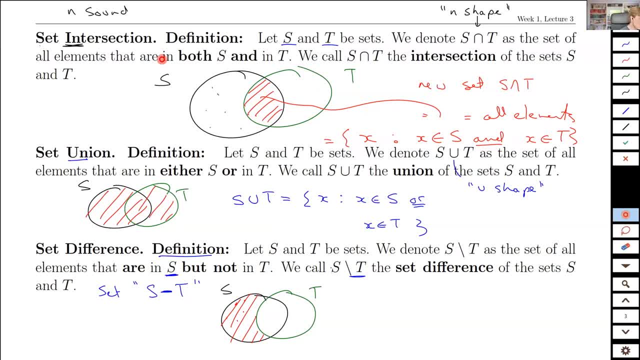 but not quite because it's not quite symmetric. Basically those three things- intersection and union being the two most important, and set difference being something you might use honestly more in computation. Just saw Madison's comment. If anyone else is having some difficulty with video lag, please do let me know. 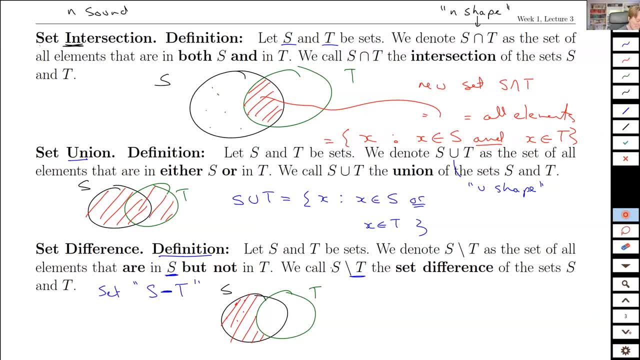 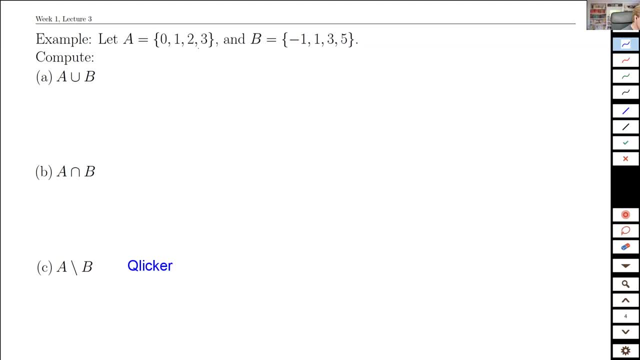 It looks fine on my end, but I'm right beside myself. All right, All right. So let's just do a quick example. So we've got the two sets 0, 1,, 2, 3, and these ones. 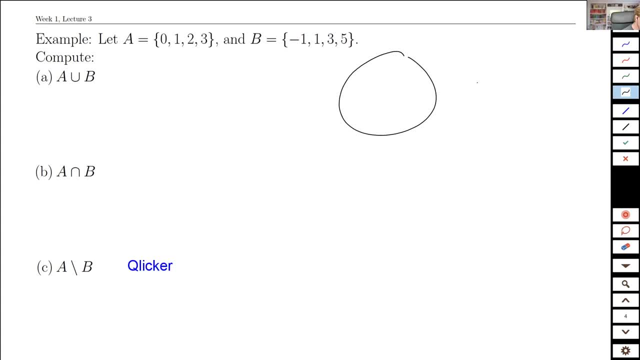 In fact, maybe it couldn't hurt this first time just to draw them out, to represent them using a Venn diagram. That's right. this is B this time, And so each one of these values, we can say, well, is it an A and B or just one of the other? 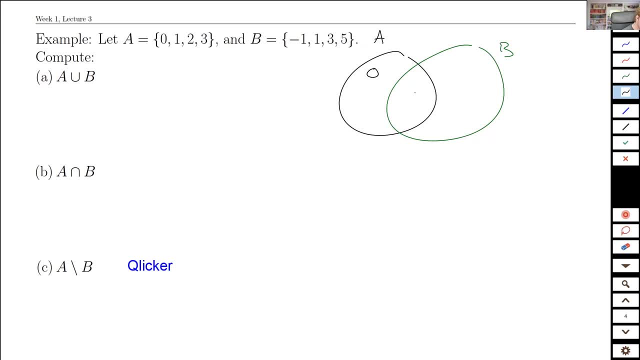 And 0 is only an A, 1 is actually in both, 2 is in A, only 0 in B, And 3 is in both And minus 1 is over here: 1,, 3, and 5.. 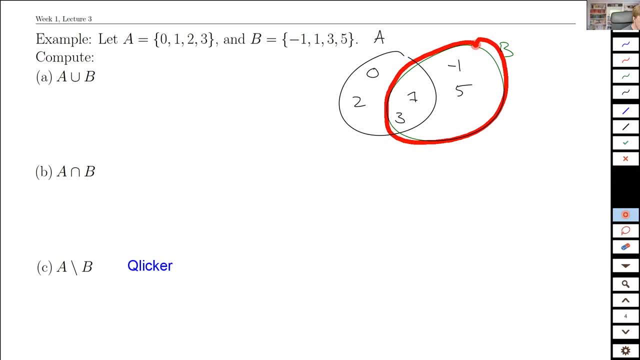 Perfect. So for those who haven't used Venn diagrams as much here, I hope it makes it a little more easy to see. The set B has four elements in it. There it is, And so inside the circle of B there's four numbers. 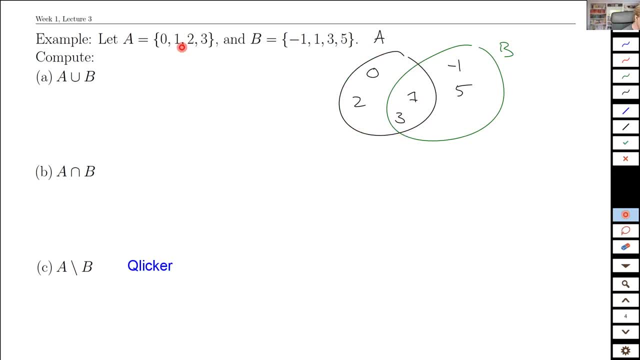 But two of them are shared with the set of A, because A also has four numbers. That's fine. There's four numbers in that set, But the overlap region has 1 and 3 in it. Just to indicate they're shared by both sets. 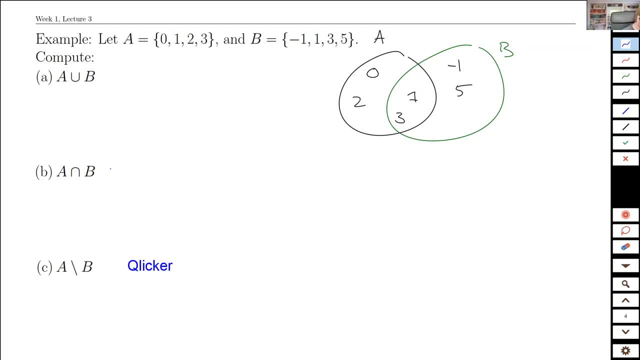 In fact, that actually gets straight to the intersection, which is what's in that overlapping region? Well, 1 and 3. If we take the union again, that's the set of elements that are in either A or B, And so that gives us an exhaustive list. 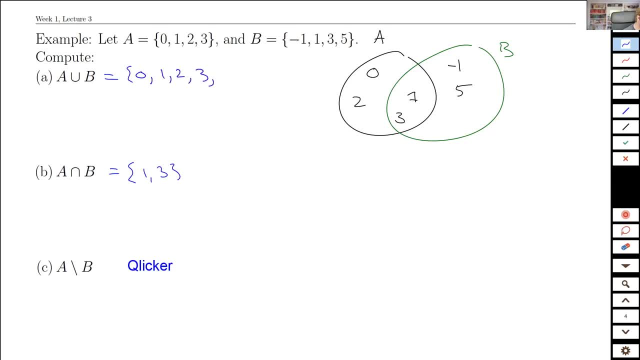 I'm just going to go through here: 0,, 1,, 2, 3, minus 1.. We already have a 1.. You could put it if you want, It doesn't really matter, But usually we wouldn't duplicate if we know it's a duplicate. 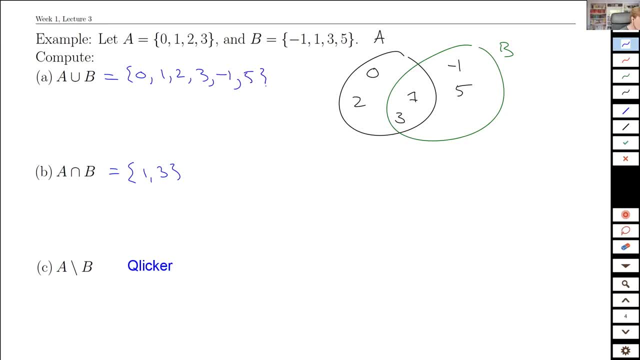 3 is also in there already And 5 is in there already. Sorry, 5 is not in there, So we have to add it, And we can see that there's six elements here, And that corresponds perfectly to how many elements we get if we count up the number. 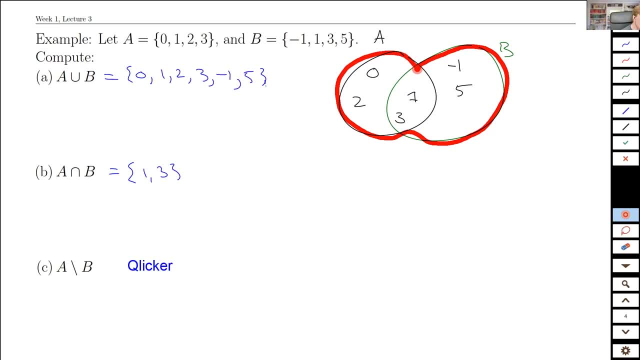 of values in this Venn diagram. There's six individual numbers, six unique numbers in that diagram, And that's what we see in the union there And the intersection is just this region here, the set of values that are shared, And both. 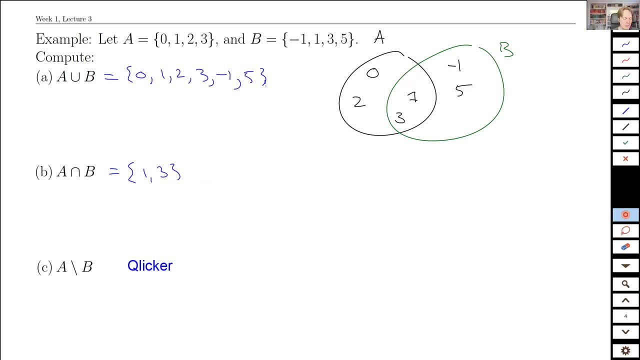 And just for fun, I've set up a clicker question for the last problem here So you can try the difference And remember. the difference is Well, I'm not going to draw it because that was the answer, But yeah. 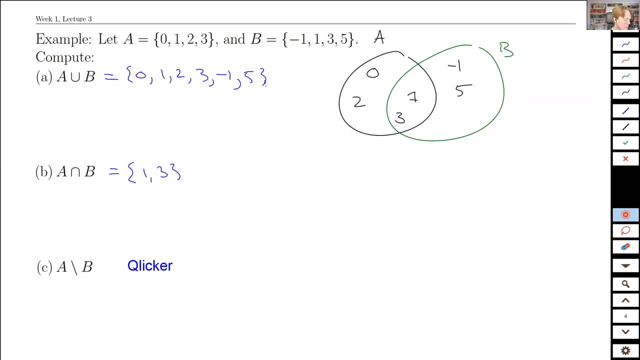 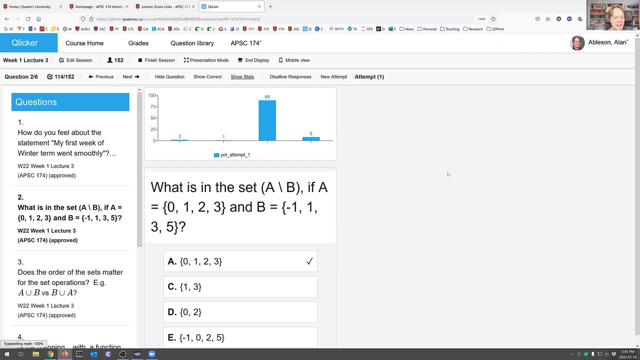 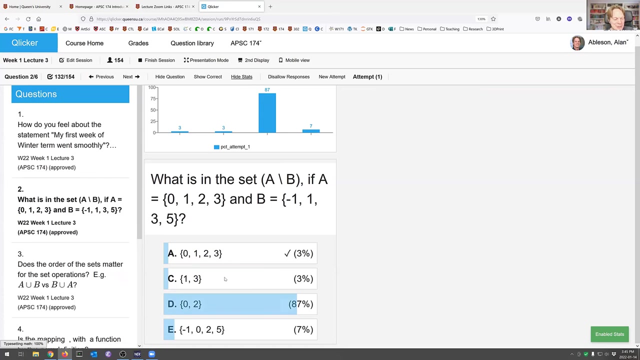 What would the difference be? A difference with B, in this case, here, Perfect. All right, I won't belabor that, But I'll just flip over to the results so you can see them. Yeah, So we're strongly there on D, which is perfect, because D is the 0, 2.. 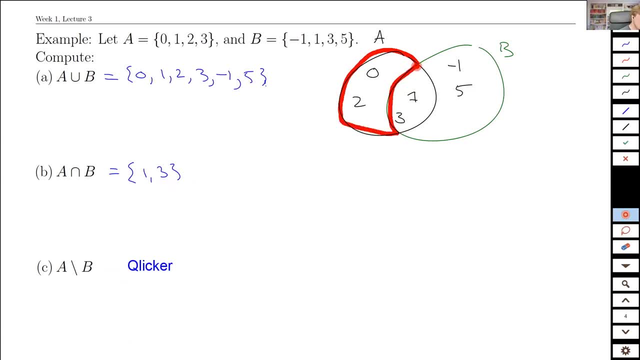 And again the A without B. so taking out all elements that are in B leaves us with this little crescent in our Venn diagram, And that's just the points 0, 2.. 0 and 2.. All right. 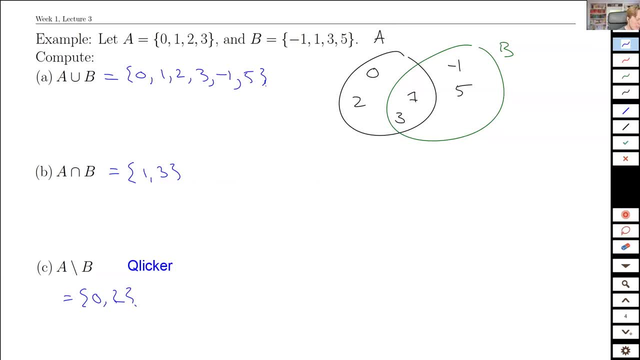 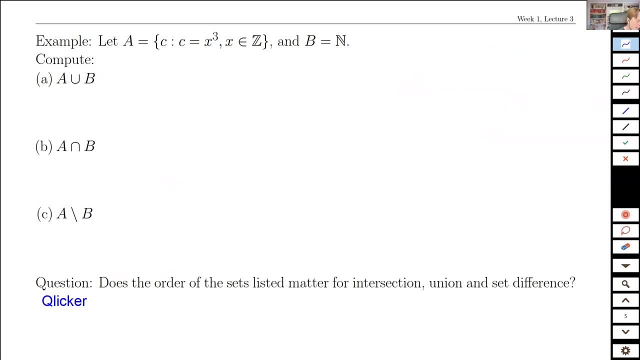 So for now, that's pretty much all we need in terms of sets. So let's go ahead and do the final test. We're going to look at the unit intersection for basic qualities. If we want to get something a little more exotic, then here's an example of that. 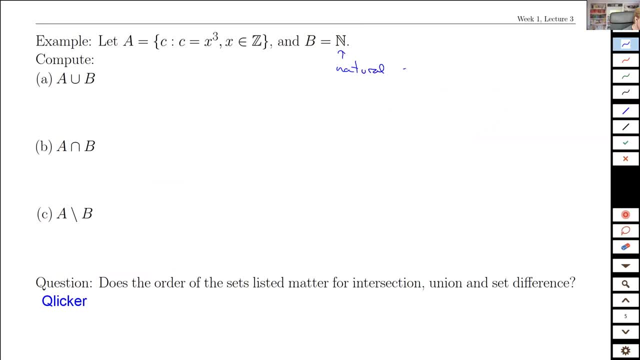 So here we've got again our natural numbers, Trying to get a new model for all these, The natural numbers, which are the 0,, 1,, 2 and up integers. Then here we have all values that are the cubes of integers. 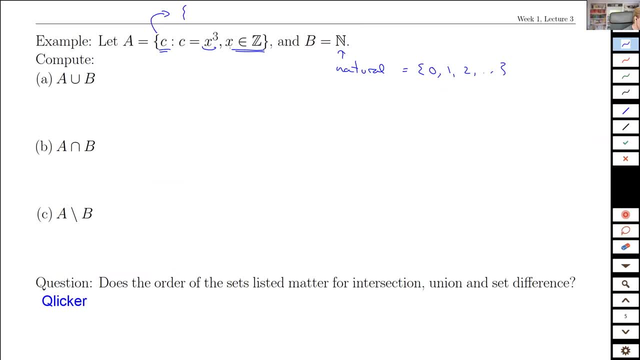 makes sense to kind of just try to describe this first. so what we can do is think about like a for loop and computation and all right. so i'm seeing hit and miss, mostly hits for quality there. all right, uh, there will be a recording afterwards and, fingers crossed, the recording should be. 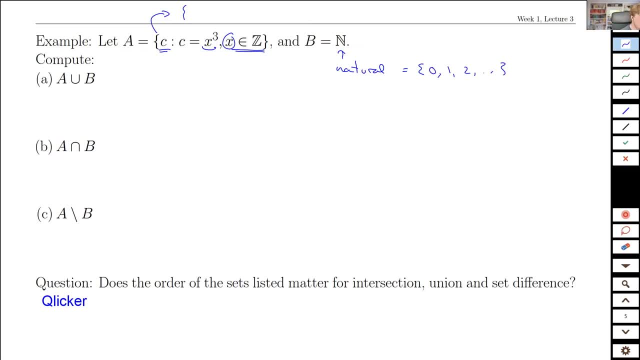 decent quality. so, um, if you are having trouble and feel like it's just so laggy, you can't even bear to watch it. i totally get that. i've bailed on things before. so, uh, if that's an issue, just wait for the recordings. we'll have them up, hopefully later on tonight. all right, so x can. 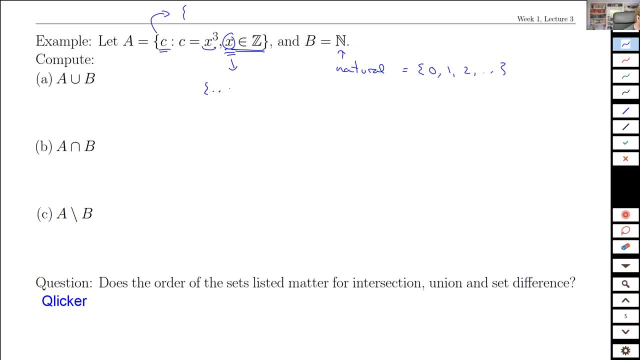 be an integer, so x can be anything from minus infinity up to these guys here. those are the x's, but we want the collection of c values, which are those cubed. so we're just going to take each of these numbers cubed and we would imagine seeing the pattern like minus three cubed is minus 27. 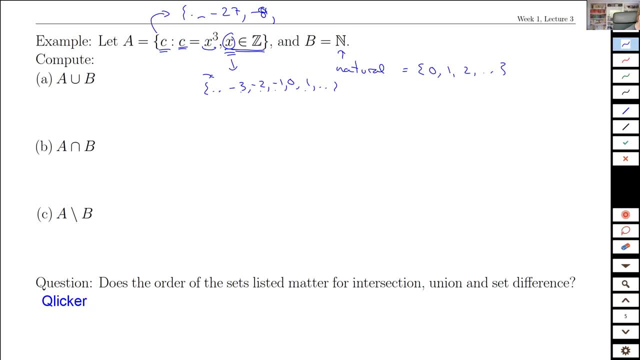 minus two cubed is minus eight, if i remember correctly, a minus one cubed is minus one, and so we'd get this pattern here again, just sort of implying the continuity down at both ends with the three dots there, and so we see these are not identical sets by any means. this is lots of numbers, but all zero. 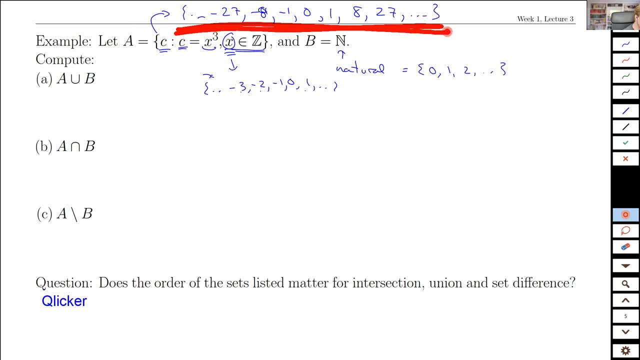 and higher. this is skipping numbers, skipping a lot of numbers, uh, but including some negative values as well, pardon me. so, honestly, i find the intersection easier to see. it's usually smaller. so here, if i take all the values that i've got, and i take all the values that i've got, 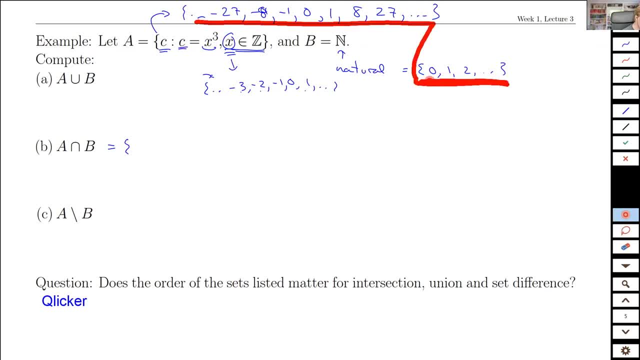 are in both of these. we are only going to get the natural numbers at most, so that rules out all of these negative things here. we're not going to get them, but zero it is in both, one is in both, eight will be in both: 27. so we're basically going to get the positive cubed values. 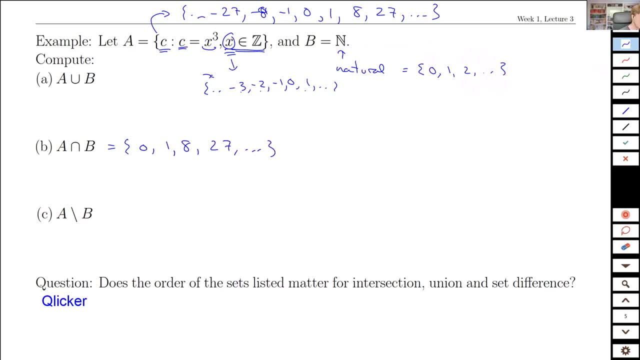 that would be the intersection, the values that are shared between both of these. where i can see it, in both sets the union is going to be a bit uglier, harder to describe, but we can imagine. well, let's start at the lower end, with the negative values, the only negative values. 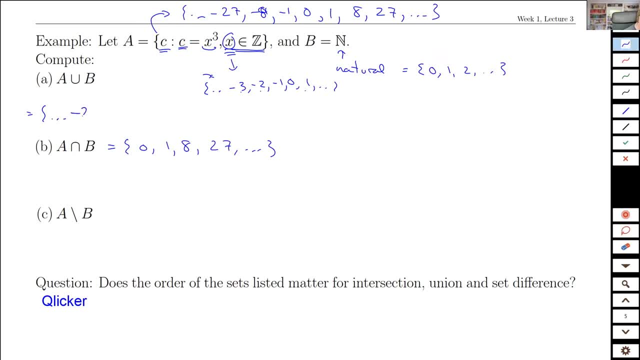 we're going to get are the negative cubes. so we're going to have a bunch of numbers and we're going to trust that the pattern implied here: decimal dot in there, negative, eight, negative one and zero, and once we hit zero, we are taking values that are in either set. well, the number. 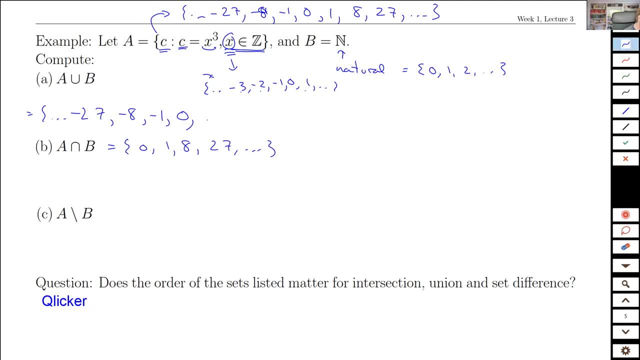 one's in this set, the number two's in this, the number three. so in the union we're going to find all the positive integers from there on in. so we'd have the negative cubes, the zero and then all positive integers after that, when we take a union of those two sets. and last but not least, 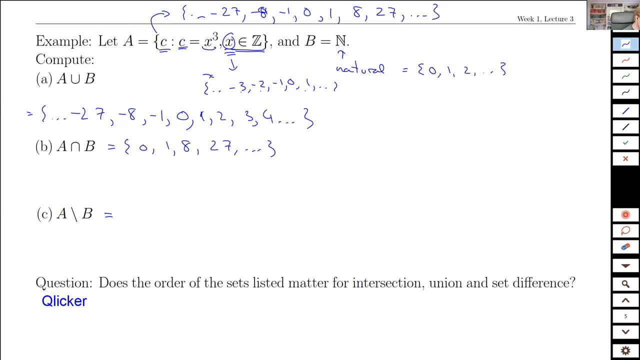 a without b. that's interesting option. so we're going to take all of these values here and subtract or remove any values that might be positive integers or zero. oh well, i'm going to take out anything that's a positive integer. that would be all these guys and that's just going to leave the negative, the negative. 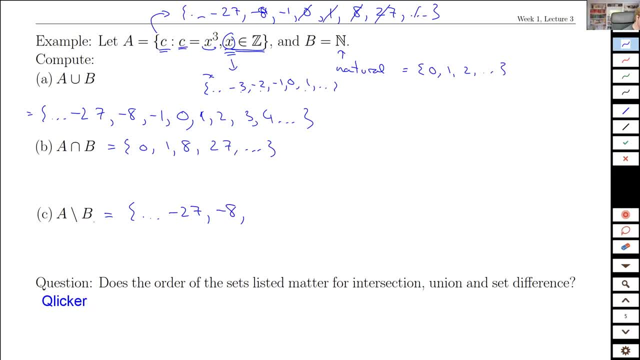 cubes in our set. for this set difference calculation here: negative one, and that would be. we would stop there this time there's no dot dot dot. negative one would be the last number, because zero is in both and we're going to remove anything that's in our natural number set. 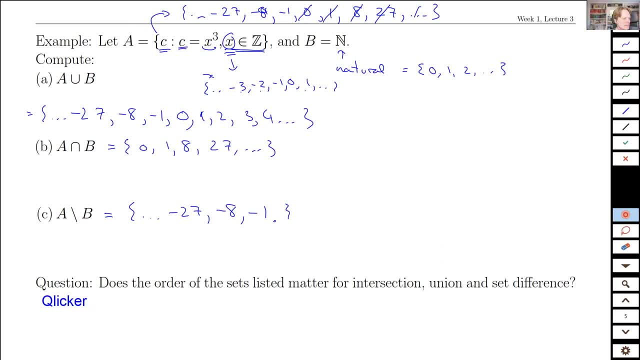 all right. so if that's the case, then think about whether these things are where their order matters, and what i mean by that is if you do a intersect b or b intersect a, if you do a without b or b without a. think about that. you get the same thing either way. 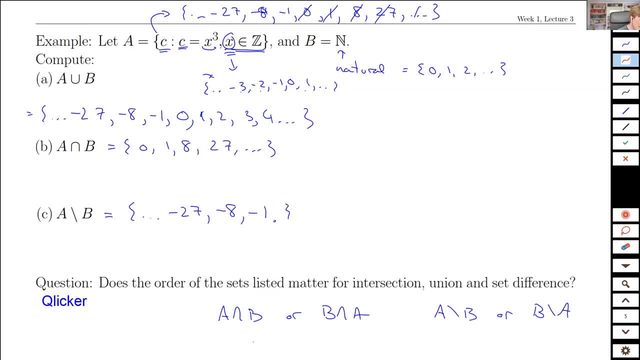 and for those who have gotten a little fancier: uh, this is about our but ativity, which is going to come up next week. can i switch the order? change the order? change the order without changing value? changing value? all right, let me just flip over to the clicker thing here. 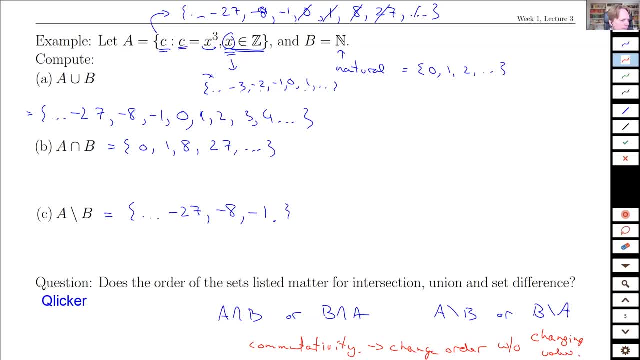 Yeah. so just one question there: Why don't we cube the integers in the union? Because the union over here is anything that's in either one. So if I say is zero in either one, yes, it is, that's in both, one's in both. 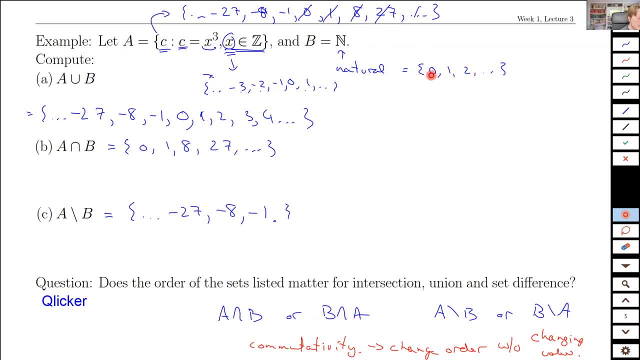 Is two in one or the other. Yeah, two is in there, So I do include two in the union. And then I look at three and go, yeah, three is in the union because it's in the natural numbers And pretty soon you realize, well, this is going to cover all my cases for the positive. 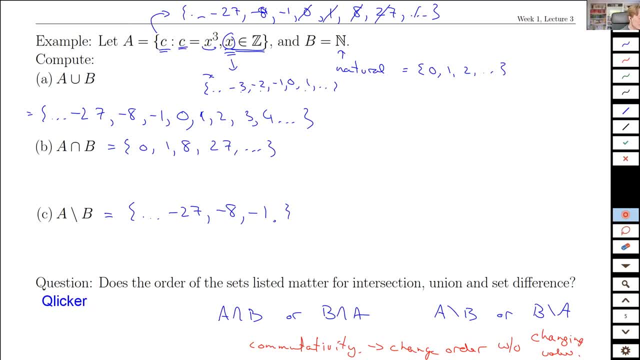 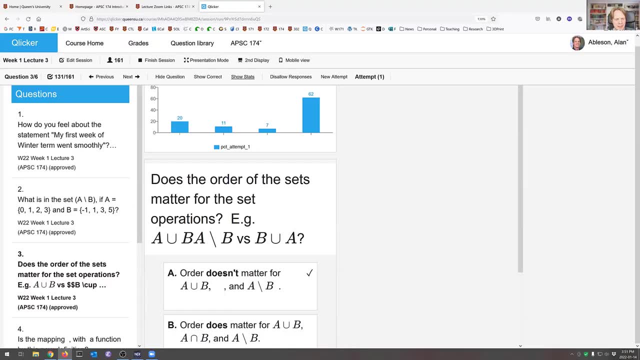 numbers. I don't have to look at the one up here. This is going to cover all positive integers. They're going to be in my union. All right, let's flip over to the stats here. Okay, not too shabby. 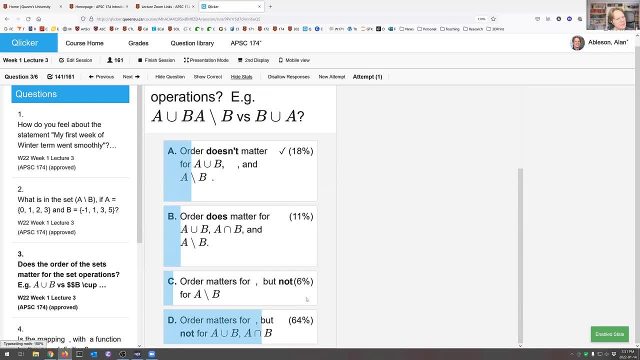 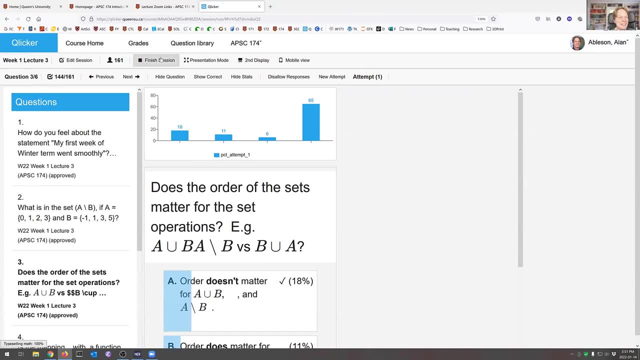 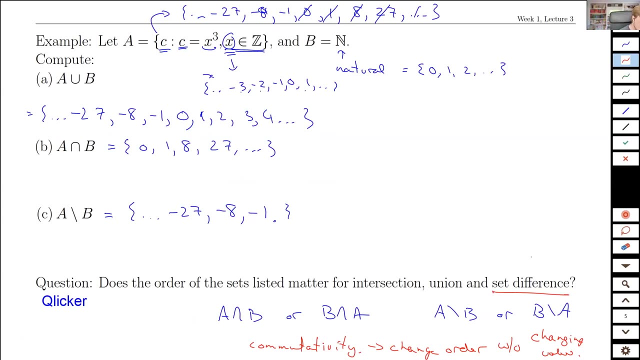 So the order matters? Oh, it looked much better on my screen. The intersections are supposed to be in there. Math notation's hard. What can I tell you? So, yes, it matters for the set difference. So for the set difference it does matter. 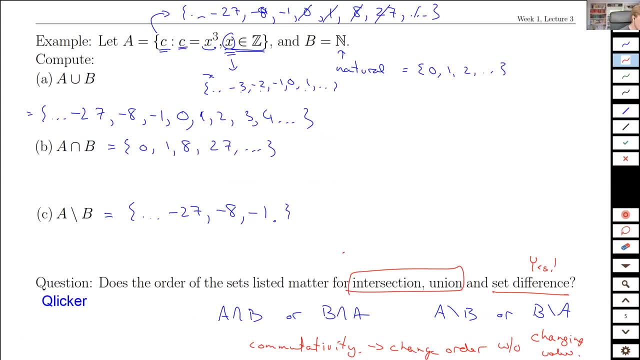 For the set union and intersection. either way is fine. So A intersect B is exactly the same as B intersect A, And likewise A union B is the same as B union A, So it wouldn't have mattered Which one. Which are these things? we call the first set if we're doing unions and intersections. 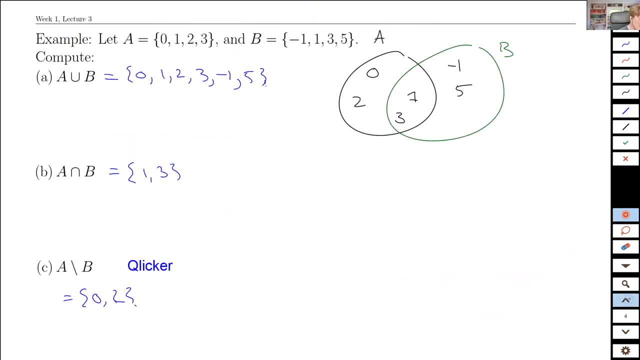 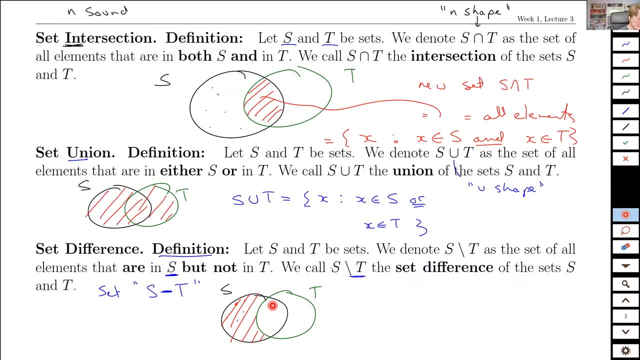 It does make a difference when we do the order, And you can kind of see that in the pictures back here right. This set difference. we got one half of this, So it mattered whether you put S or T in there, because we only got S elements left over. 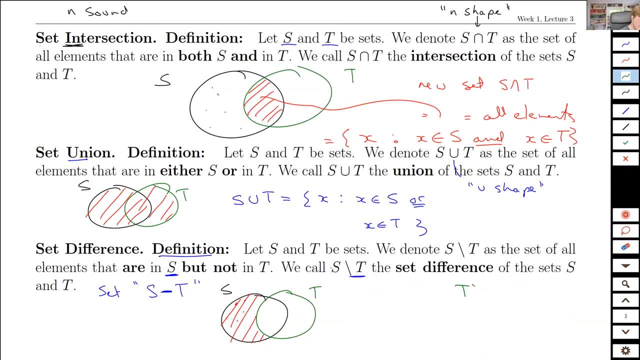 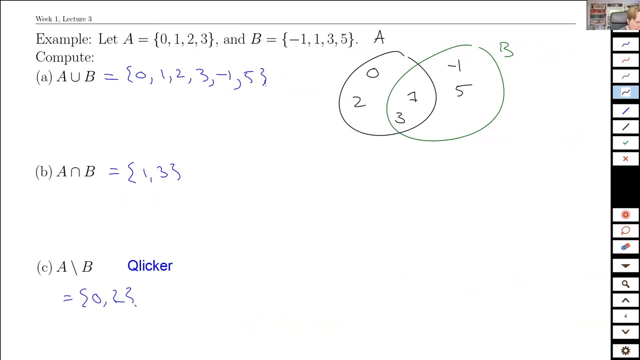 This part over here. if we did T difference with S, that would have been everything that's in T but not in S. I just realized I'm going to disable these things. S and T, yeah. So there, it does make a difference which order you do them in. 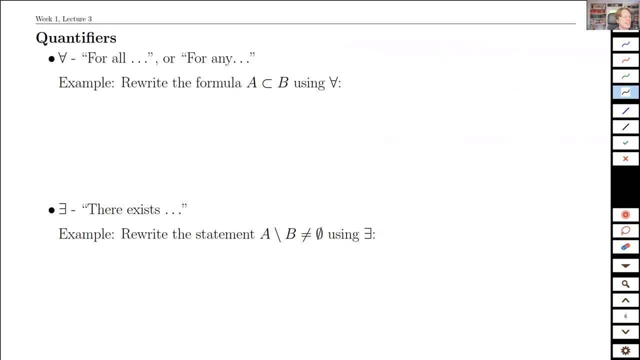 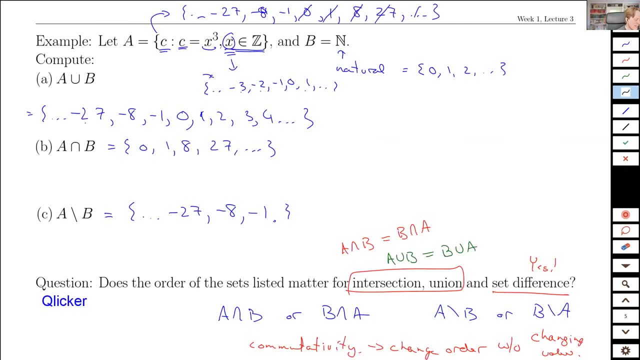 For sets. honestly, we don't do a whole lot of work with sets that are infinite, especially because it gets really dicey to get into the minutiae. how do you actually write these things out without just kind of waving your hands with dot dot dots? 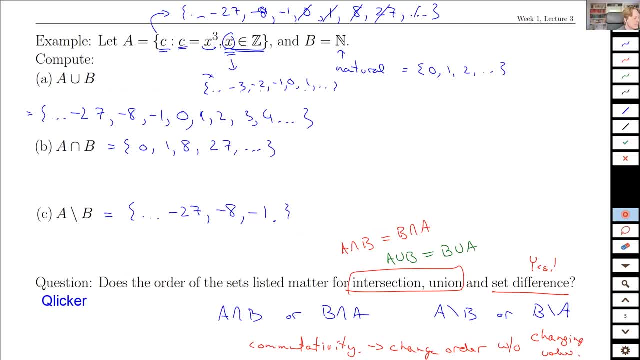 So for now, For now, as long as you're understanding the concepts, that'll be fine. The best test for whether you've kind of got a good handle on this is the tutorial problems and the web work, which typically deal with finite sets, to avoid this kind of messy notation. 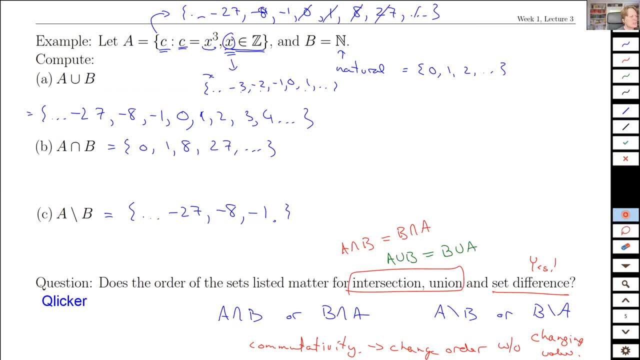 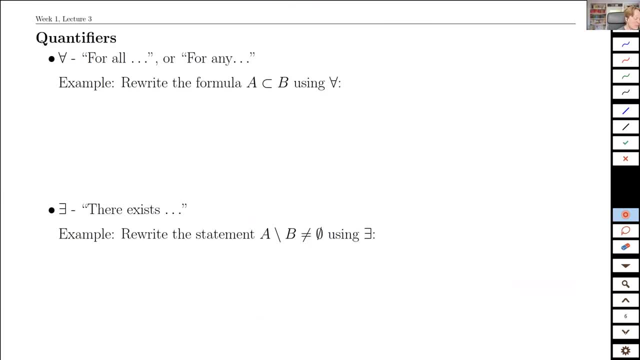 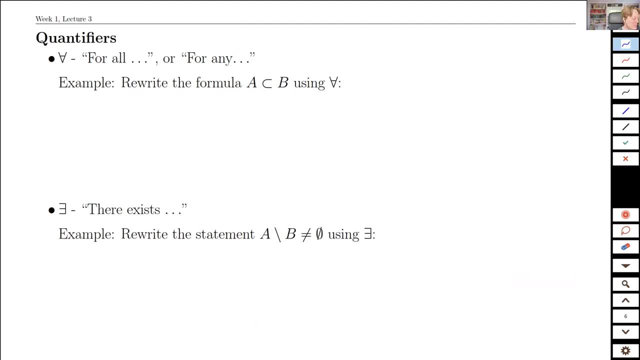 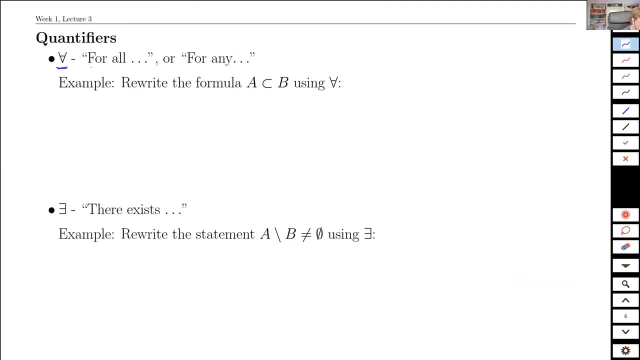 So here they are. The upside down. A is read as for all or for any, and the idea is that we can maybe rewrite some of these intuitive statements. It's like the intersection statement or the subset statement, and using these kinds of terms, 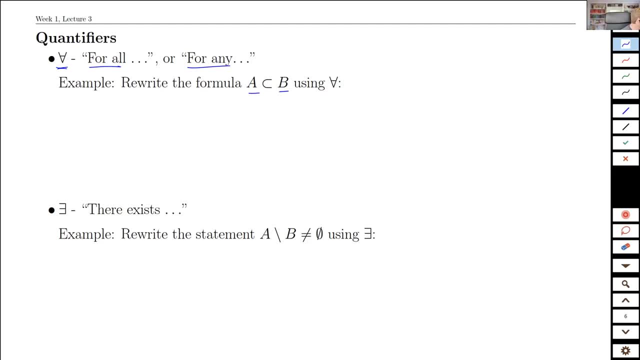 Sorry, I'm just trying to bring up my own notes here for a second. So the way the subset notation works is: if A is a subset in B, then any element in A, any element X in A- let's put that a little more clearly, my apologies- is also in B. 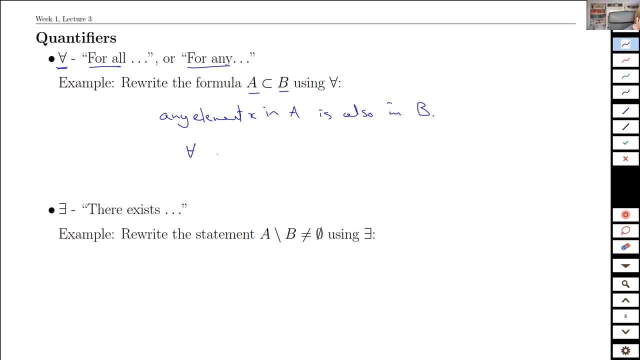 So one of the things that we can say, that is, for any element X that is in A, we get the implication or the results, or it implies that. it implies that that X is in B. That's right, That's implied here also. 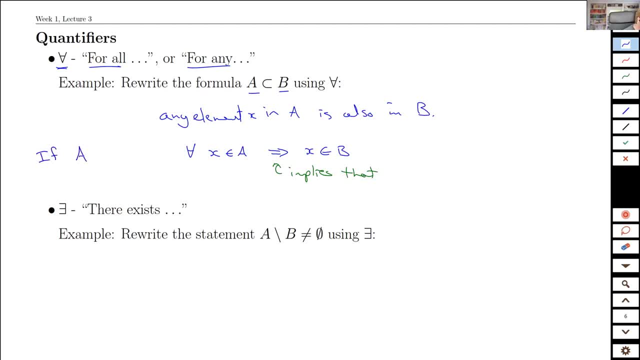 So there'll be a statement here: If A is a subset of B, then for any X at all, no matter what X I pick, that's in A, I'm guaranteed that that X is also in B. So that's kind of how we use that. that for all thing. 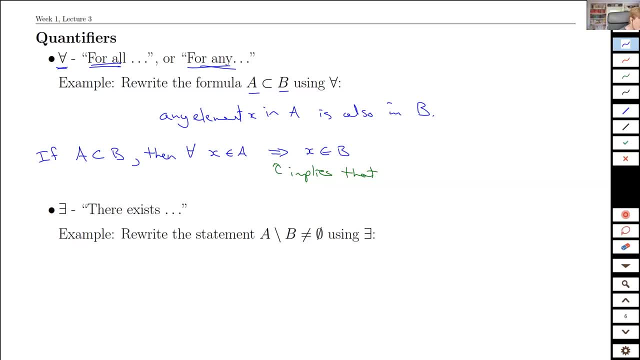 That's one of the examples, But think of this for all or for any, in terms of how you say it out loud. Then there's this backward, There's this E that has this for there exists. So think about the statement here. for a second: A minus B is not zero. 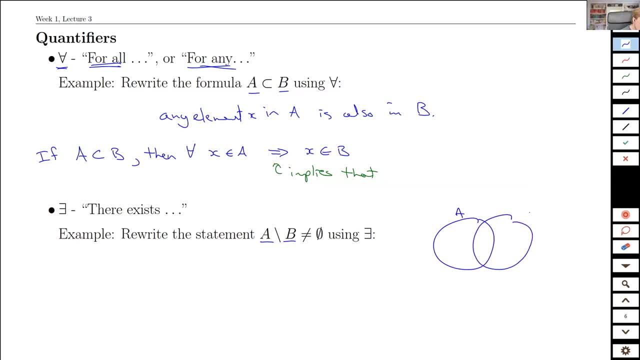 So let's just draw this little set here. So if I draw A and I draw B, and let me imagine what would I get if I had it equaling zero. So if I have A and then maybe B is like this: A and B In this case, here if I take A, but 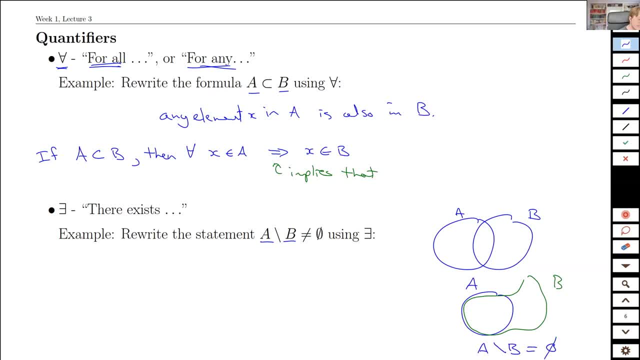 then I subtract everything that's also in B, I would get the empty set right, Whereas up here A, if I subtract B, I don't get the empty set. That's sort of the two scenarios here. There's something in A that's not in B as well. 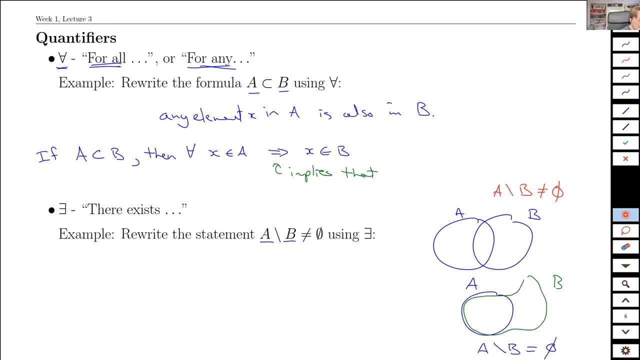 Here everything in A. unfortunately, it's also subsumed by B as well. Unfortunately, it just happens to be the way it is. Well, that means there's something in this part here, this little crescent shaped thing that we saw before. 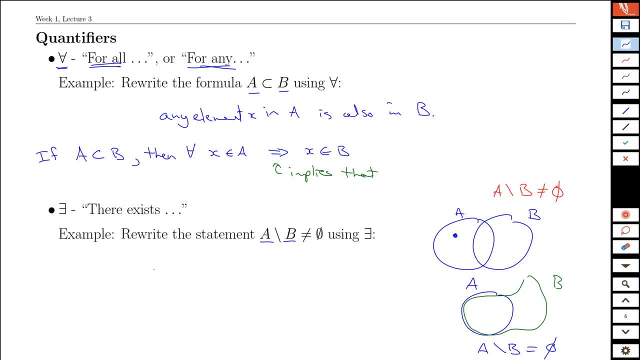 There is an element in there. Oh, that means if A slash B is not equal to the empty set, then there exists an X value that's in A, but X is not an element of B. Not an element of B, In fact. there it is. 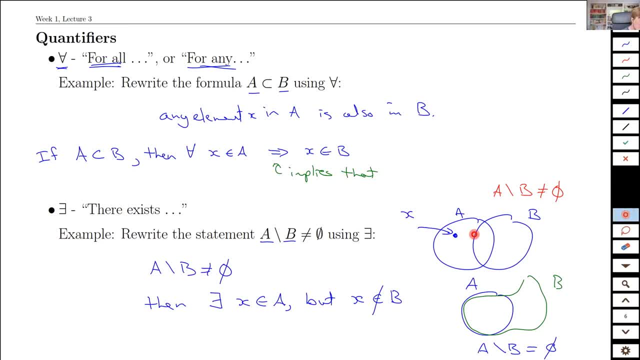 I know there's at least one thing hiding in that part of this diagram That satisfies that X is in A but it's not in B, and that's where this there exists thing symbol comes in handy. I don't know what that number is. 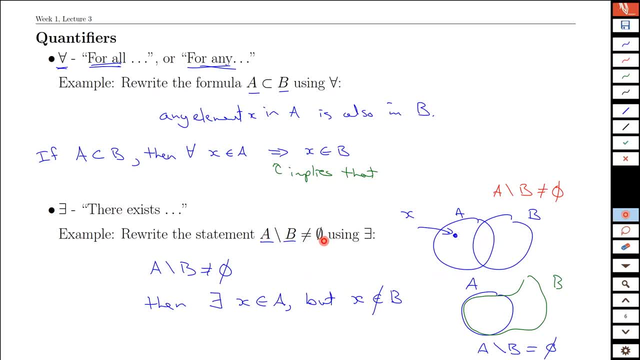 I just know that there has to be one, because we said the A slash B was not empty, So there had to be some element. There had to exist some element in A that was not being deleted when we subtracted B. So all righty. 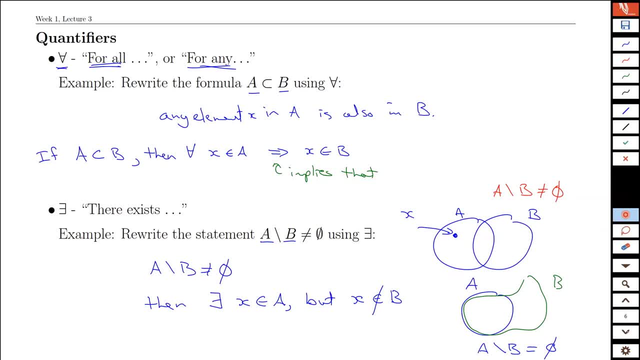 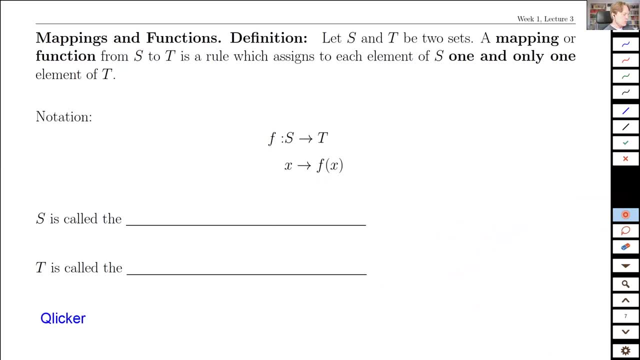 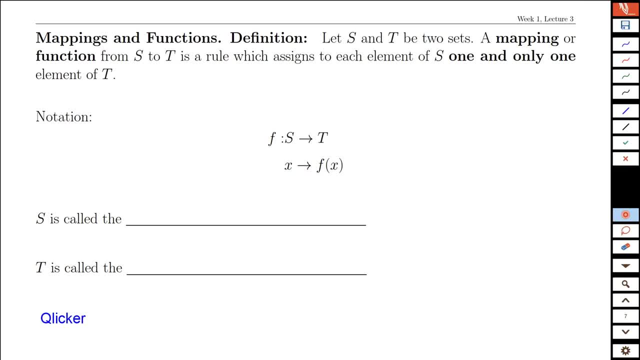 All right, I'm going to have to pick up the pace a little bit. I apologize, All right, This is the key stuff for this class, For this lecture is mappings and functions. So we are going to tweak just a little bit the definition that we're using for functions. 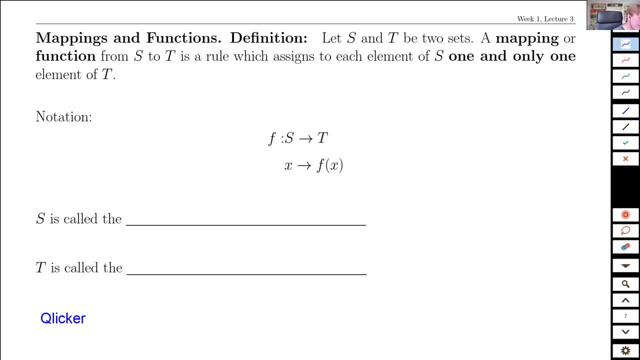 compared to what you've seen in calculus and previous math courses, And one part of it is stuff you have seen. So we're going to map now from one set to another set. So now we have two sets at play right now. Up until now we just had one set and it was kind of hanging out by itself or maybe intersection, that kind of thing. 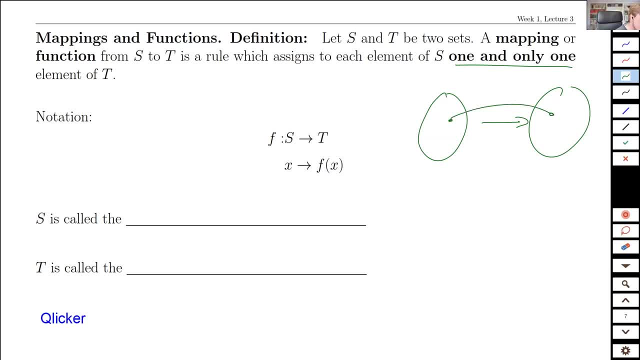 But now we're going to take values in one set and we're going to map them to a value in the other set. So here in rs and t, And our function is: what's doing this? Now the output value here. this is like calculus. 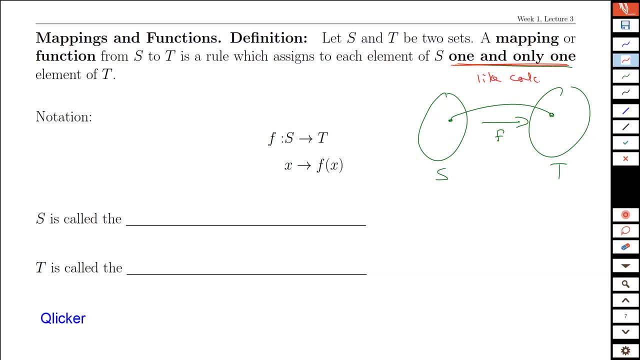 Like calculus. Like calculus, If you have an input value, you only have one output value. You don't have one input going to two output values. So it's like you can't have x going to y1 and y2.. That is very important. 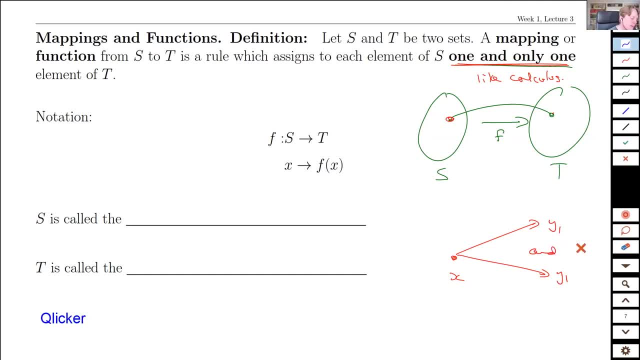 That's a big x Functions don't do that. They never have. What's new here, And perhaps a bit annoying, Is the each element here. This is new. This means that every element in the input set has a defined output. 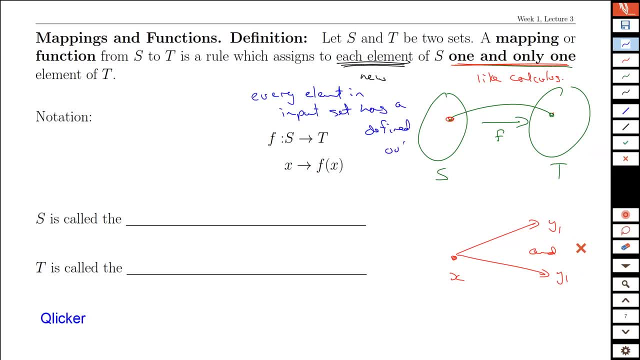 Has a defined output, And we're going to go through some examples showing why does this cause grief, Especially in calculus type functions. So In this case- here we've got some nice names- S is called, not surprisingly, the input set. 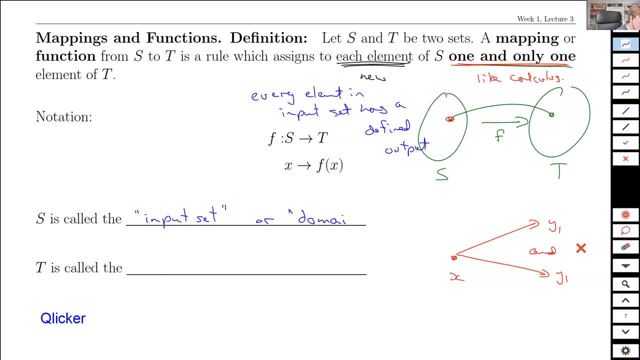 Or sometimes, using more calculus type terminology, the domain set T, of course, would be the output set Or the target set. We try to avoid the word range, which might be something you go for, Because it's not the range. 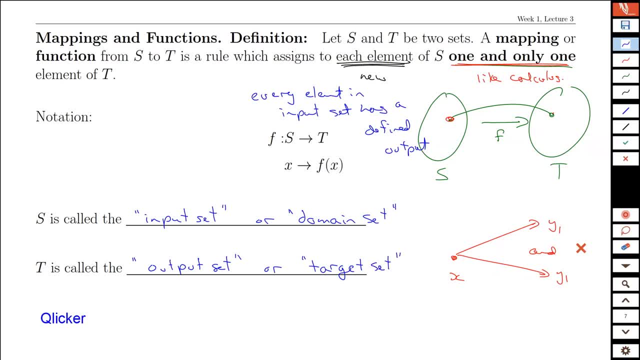 But it's the format Exactly, As we'll see through some examples. All right, Let me just pause there. This format here is a little more explicit than what we've done with describing functions before, So usually we would have just said f of x equals like x cubed. 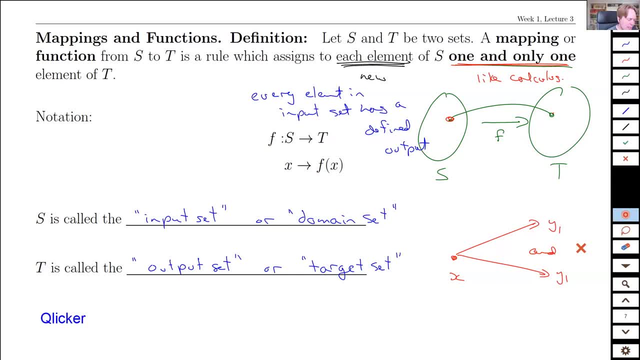 Something like that. But when we take a look at this new version where we're explicitly defining the sets, I think you'll see there's some subtle shading that comes in with that, But it helps to actually make things a little clearer Or at least more transparent about what's happening. 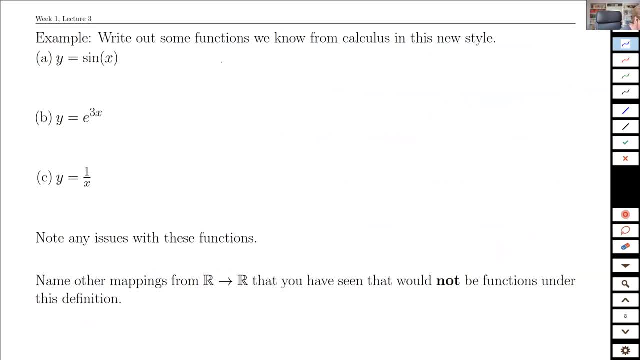 So let's take things that we know: Y equals sine of x. We would write that now, as f is a function that maps from the reals to the reals, And every x gets mapped to sine of x. All right, So in some sense not a big deal. 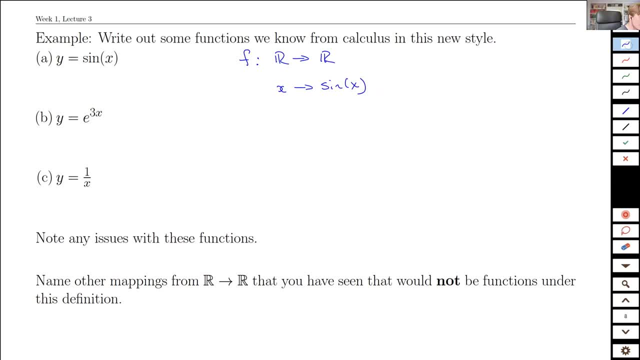 It's just explicitly saying what the input and the output values are, And you can think back to 171, where we had, you know, functions of time that mapped to, or even 172. now, When you're going around the ellipse, you had values of time and parameterized curves where you got x's and y's back. 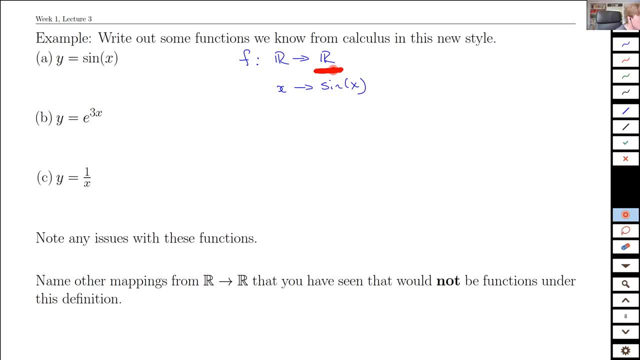 This is a nice way to encapsulate that and say no, no, no. Okay, We've got real inputs and maybe two-dimensional outputs. We would have had R2 there. Let's stick with 1D for today, though, One variable functions. 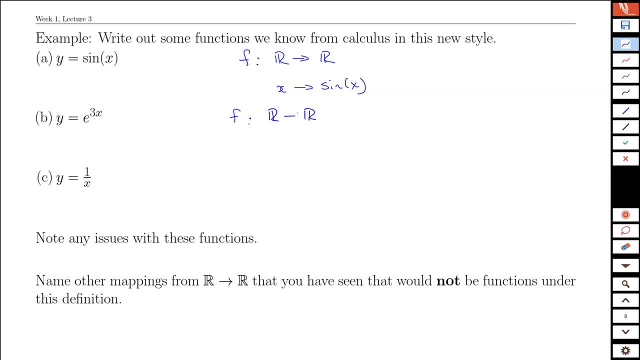 Here we would have the same kind of thing. I'm going to map real numbers to real numbers. The function is e to the 3x. That's fine, And every x is going to get one e to the 3x value back. 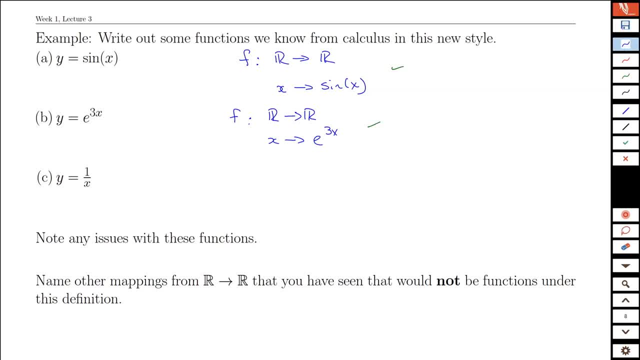 So that's fine. These are both great. Where we get into some wrinkles is this example here. So if we claim this is the case, x goes to 1 over x. If you think about domains and these kinds of questions and the fact that domain came up so explicitly, this is actually a problem because 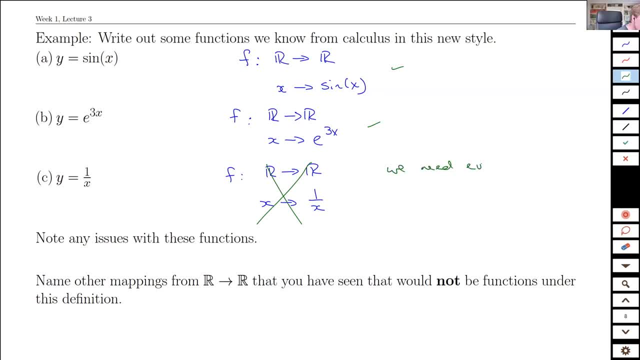 We need every input, Input x, to have a defined output. Defined output- And where's the problem with this? But 0 in this function maps to 1 over 0, which is not an element of the reals. So, basically, this is not a function. 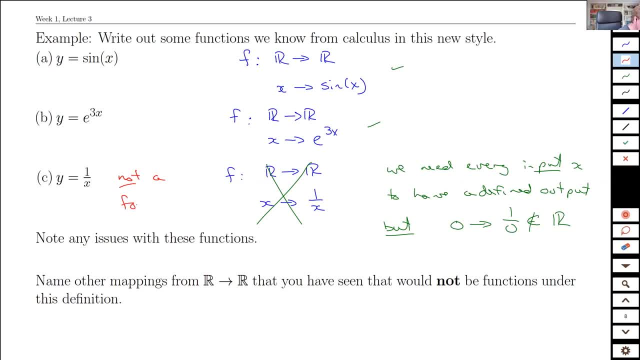 This is not a function. This is not a function, But here's where it comes handy. It's not a function on the reals to the reals. So just for a second here you might go. but if you're calling it a function all year for the last two years, when was the last time you saw 1 over x's? 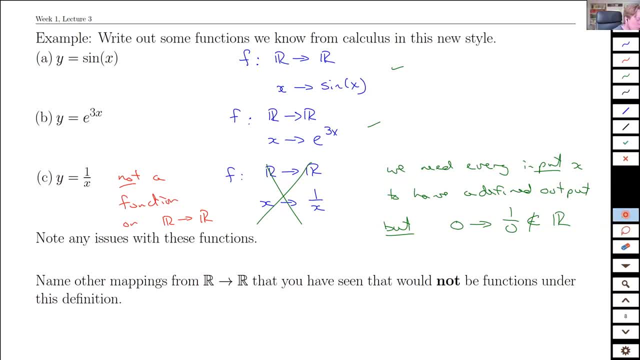 It is a function. Well, yeah, What does calculus do to get around this? We kind of hinted at in our first lecture about calculus being a pile of rules that kind of fit together and kind of make it work, Whereas linear algebra is like no, no, no, these pieces not fit perfectly. 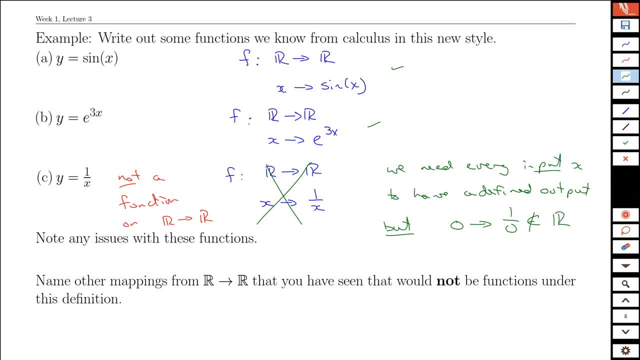 There's none of this edge case silliness going on What we do in calculus. we actually wave our hands a lot And we would say that y equals 1 over x is actually a function that maps some set s to the reals. 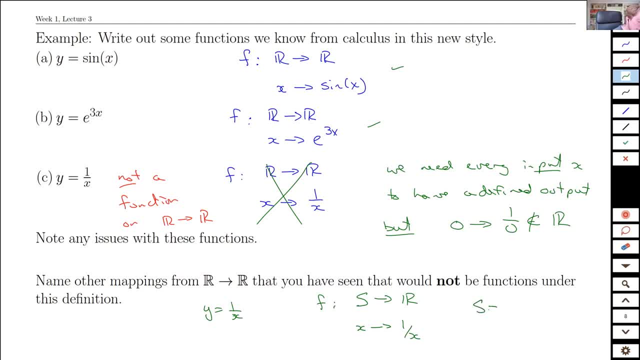 And x goes to 1 over x, Where s is equal to the set of all values, Where x is real But x is not equal to 0. Right, We talk about the domain of 1 over x and say, well, yeah, yeah, yeah. 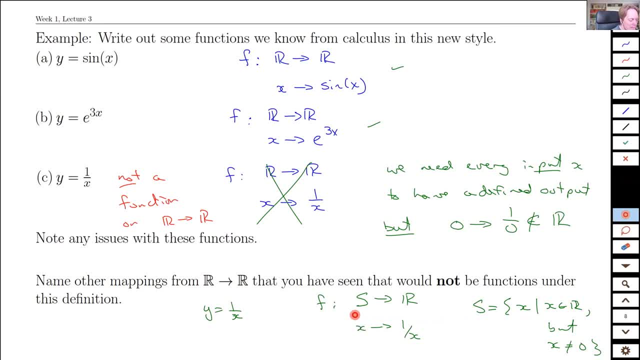 We know that you can't plug 0 into there, So we just kind of leave it out. And so this definition lets us do that, But it doesn't let us kind of brush the issue of the bad inputs under the carpet. It says no, no, if you're going to do this, you better say where this function is defined and not cheat about it. 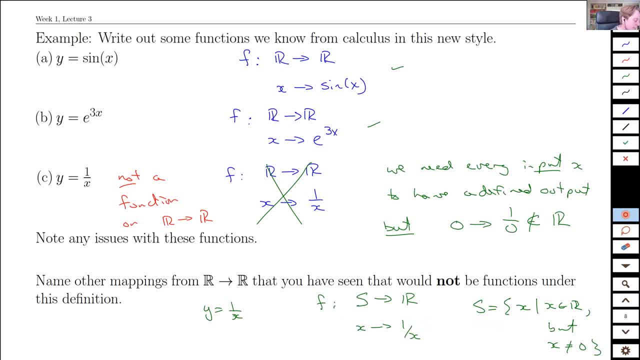 So you actually have to define: Okay, So this is a valid input set, So just be aware of that. So a lot of the functions that we know and love are exactly what you'd expect in this new notation. Any time there's an asymptote or an undefined point or undefined interval, their linear algebra is going to ask us to get fussier and say, yeah, well, on what set are you actually allowed to send? 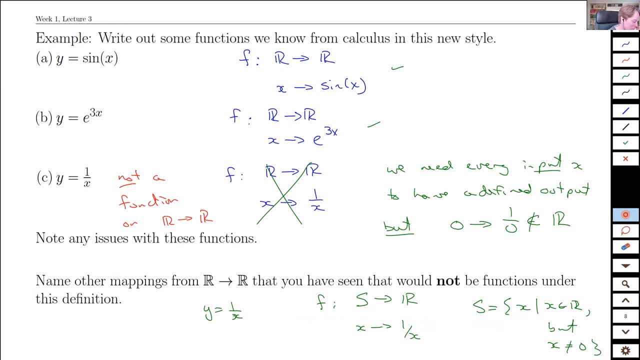 What set are you actually going to use as the input set? What are you excluding from that here, like the value 0 for the function 1 over x? Of course, that leads to a whole pile of other things that would not be functions. 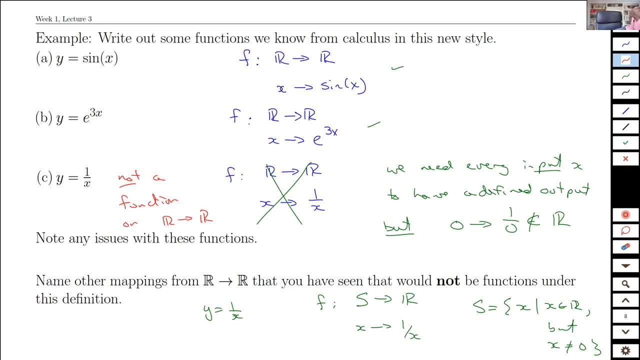 I had a clicker question but I think we'll skip that in the interest of time. But you can imagine anything that has an asymptote, So like: tan of x is not a function because of its asymptotes. Lon of x isn't defined for negative numbers. 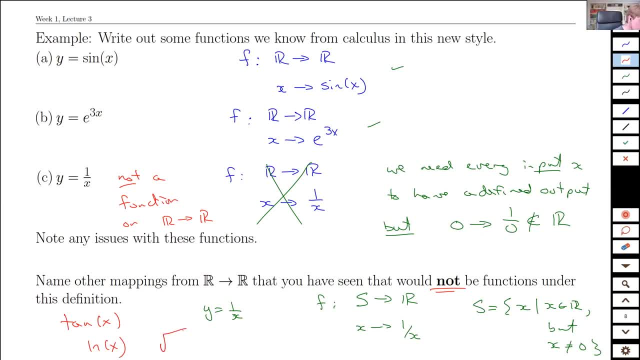 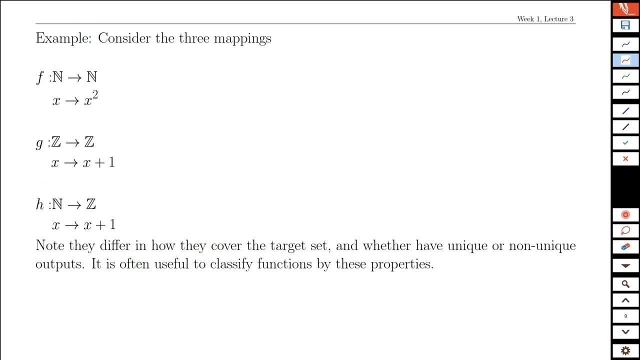 This might be a good chunk of it. What else? Oh, square roots, Square roots with real numbers. Square root of x isn't defined for negative numbers, Things like that. Okay, Can we get a little more exotic, like mix and match what we do with our functions here and our other new kinds of sets, like our natural numbers and our integers? 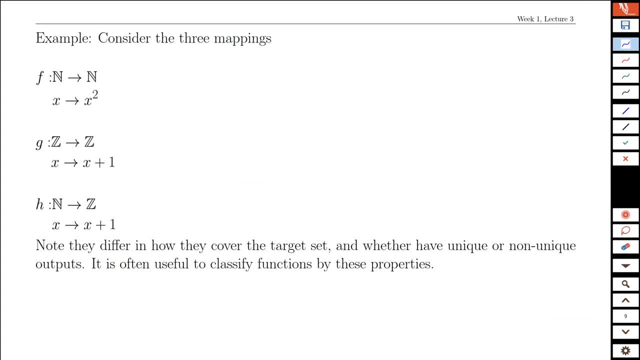 Absolutely So sorry. what am I going to do here? Right, If we map the natural numbers to the natural numbers with a squared function, we might ask: what is the range? This time we'll use the range Equals the part of the target set that is reached. 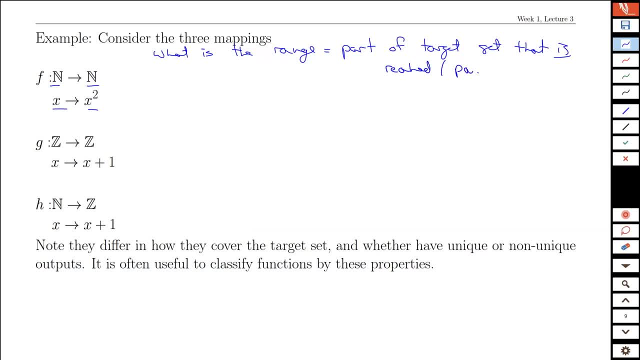 Reached- And by reached I mean part of the output- So many voices, Or mapped to by at least one input. Okay, All right, All right, Let's see what I mean here when I actually do this. There's a lot of words to say. 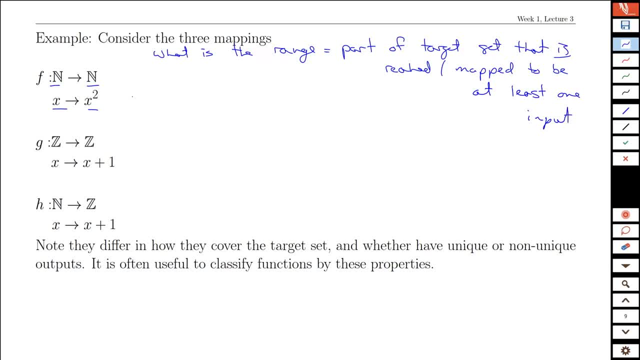 What values do you get back out? So the range set for this is going to be- imagine, taking all natural numbers, So the input 0, 1,, 2,, 3, and so on, And if we square it, the output is going to be 0,, 1,, 4,, 9,, 16, and so on. 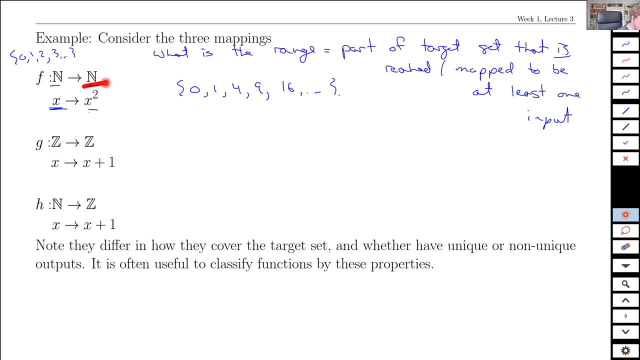 And that looks perfectly valid. We took natural numbers in. We get some. The rule about having to cover everything is not required for the output, It's just for the input. But every input has a single output, Every single integer I put into this squaring function gives me a new 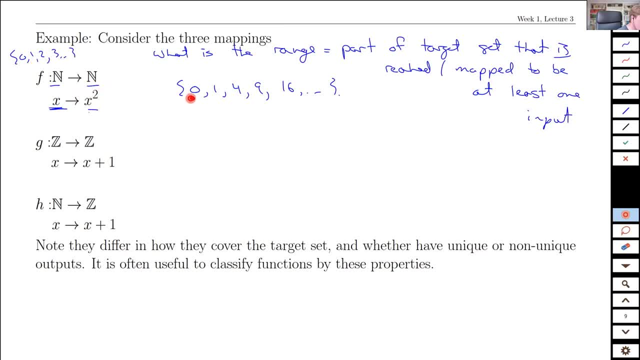 Sorry, Every natural number I put in gives me a natural number back, And we can do similar things with the integers, like this: Up to minus 2, minus 1, 0, 1, 2.. When we run those through the function, we get the same numbers. Well, actually we get the same numbers back, except plus 1.. So we'd have like a bunch of numbers minus 1, 0,, 1,, 2,, 3,, 4,, 5,, 6,, 7,, 8,, 9,, 10,, 11,, 12,. 13,, 12,, 13,, 14,, 15,, 16,, 17,, 18,, 19,, 20,, 21,, 22,, 23,, 24,, 25,, 26,, 27,, 28,, 29,, 30,, 31,. 31,, 32,, 34,, 35,, 36,, 37,, 38,, 40,, 41,, 42,, 43,, 44,, 45,, 46,, 47,, 48,, 49,, 50,, 51,, 52,. 53,, 53,, 54,, 55,, 56,, 56,, 57,, 58,, 59,, 61,, 62,, 62,, 63,, 64,, 57,, 62,, 62,, 63,, 64,, 57,, 62,. 69,, 69,, 71,, 62,, 63,, 67,, 68,, 69,, 70,, 72,, 62,, 67,, 62,, 67,, 78,, 71,, 72,, 63,, 63,, 62,, 68,. 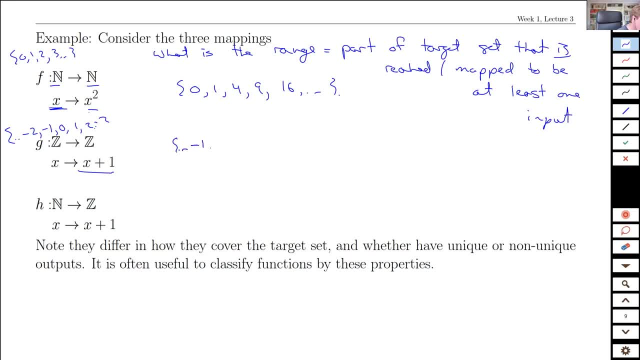 72, 69,, 79,, 78,, 72,, 63,, 62,, 69, 62.. So these are the values we put back, And we can do the similar thing with the integers like this: Up to minus 2, minus 1, 0, 1, 2.. 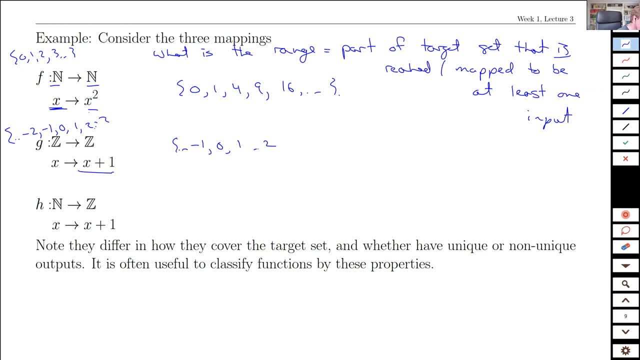 When we run those through the function, we get the same numbers. oh, actually, we get 1,, 2,, 3, and so on. So these are the ranges. this is the set of values that we get out of this function given. 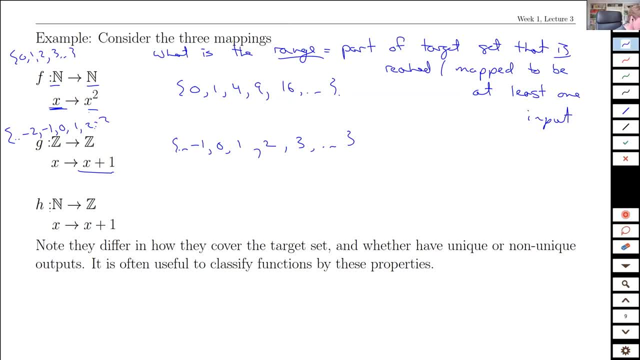 the input sets we have, And another interesting one: we can take the naturals as the inputs. so that's again starting at 0, and then finding the output if we add 1 to all of those which are in fact integers as well as natural numbers. 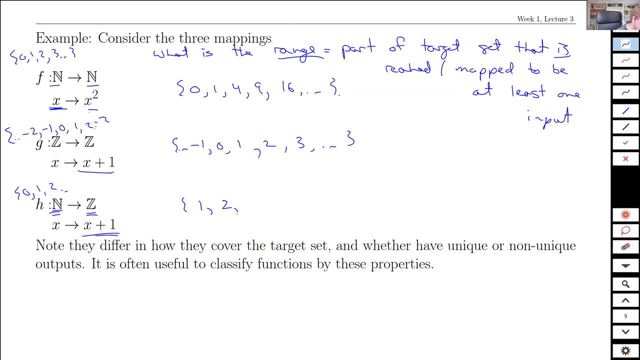 And there we get 1,, 2,, get my commas interspliced there, 4, and so on, and there we are. So we can define functions on other sets. and that's dandy, that's fine. Usually it's not that interesting. I'll be honest, most of the time we do work with the 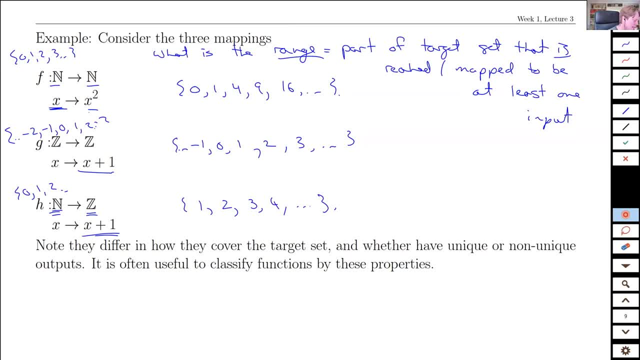 reals. But what's more interesting to me right now is actually this part. here, Actually, We actually got the same set back. So there's transformations of individual values, but there's also: what range of values do I get over if I take all the possible inputs? what kind of outputs do I get? kind of like, 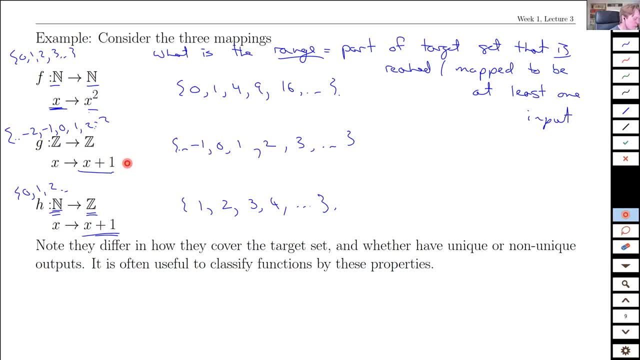 a graph, And this case here I actually reproduced the entire set. Well, that's interesting. that's different from these ones here, where I got some natural numbers, but not all of them, And it turns out this idea of having unique or not unique things is a useful way to categorize. 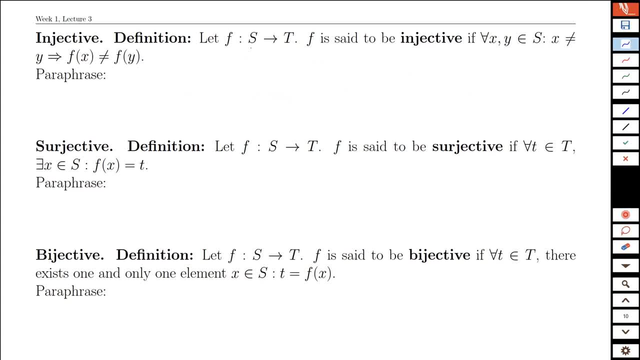 functions. So we're talking about functions again. Functions take one set into another set, And the versions we're looking at here, or the characterizations we're interested in, are called injective, surjective and bijective, And there are other ways to phrase this. in fact, these are the phrases that are used in. 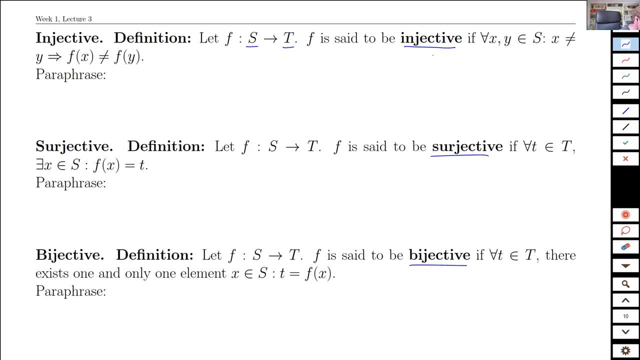 your WebWorks assignment, so I want to make sure we cover those. Injective is also called one-to-one. Let me try to write that more legibly. Injective is also called one-to-one. Let me try to write that more legibly. 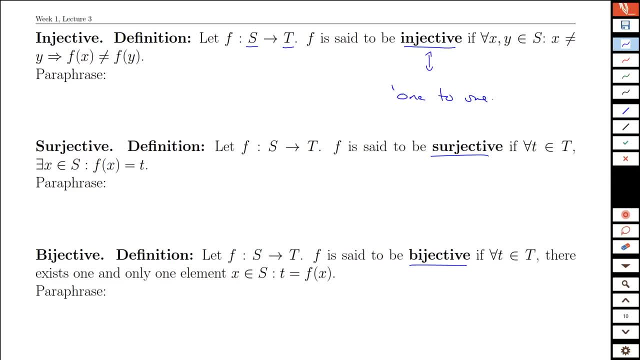 Injective is also called one-to-one. Let me try to write that more legibly: Injective is also called one-to-one. And where's the math on this? Alright, So if you have an input x and another input y, so two input values, as long as they're. 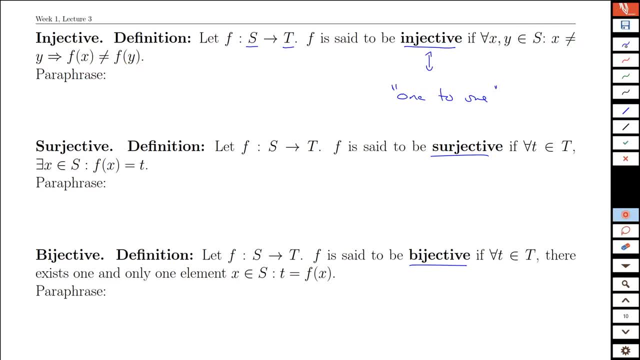 different, then we should get two different outputs. So if we pick x and y, we have to get two different values for the output. That's y, Okay, So it would be bad or not injective, not one-to-one, if we had x and y, so two different. 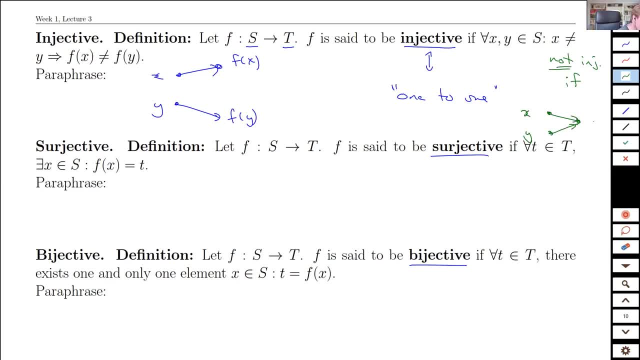 inputs that end up in the same output. That would be not injective. That's: f of x equals f of y, And this is like squareds, right? If you had minus two and plus two and you square them, you get four for both of those. 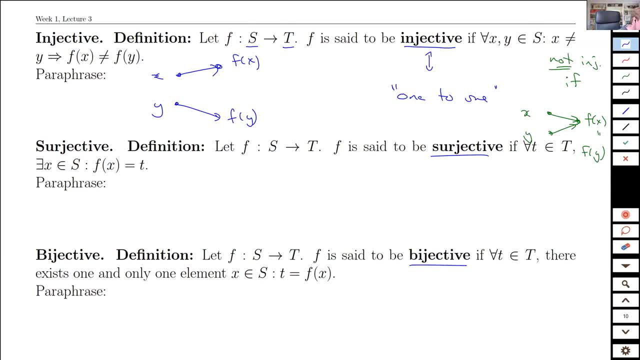 That would be something that's not injective. Surjective is also known as On-to, And you can think of this like it's. I don't know, maybe it's just the French Surjective, it's on top of. 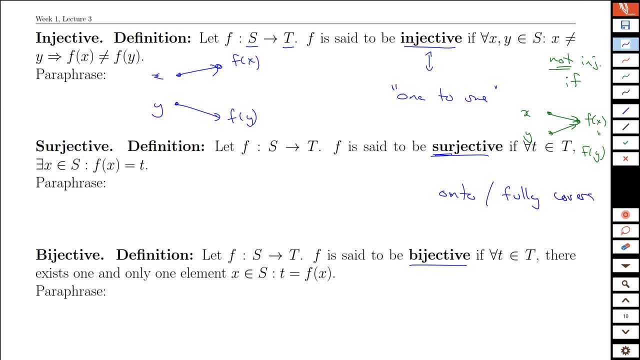 So it fully covers the output. And here we're going to get to practice: our there exists and for all. So if I take any element in the output set, so imagine you've got your sets now- if I take any element here, you can think of this as the integers if you like. so, like all. 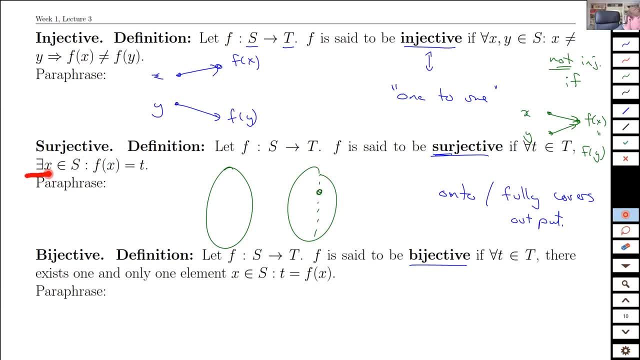 zero. You pick any one of them you like. there exists guaranteed. if this function is surjective, there exists some x in the original set over here. So you pick one random one here. you're guaranteed there's going to be an x on the other side. 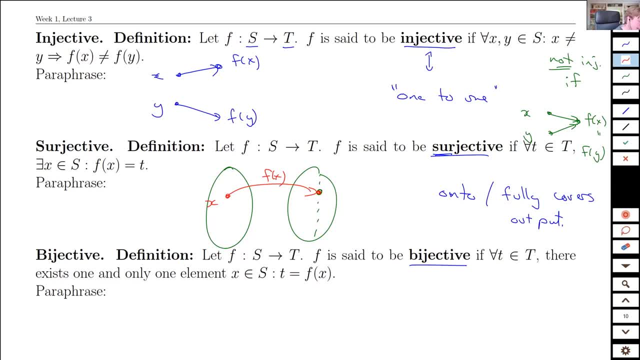 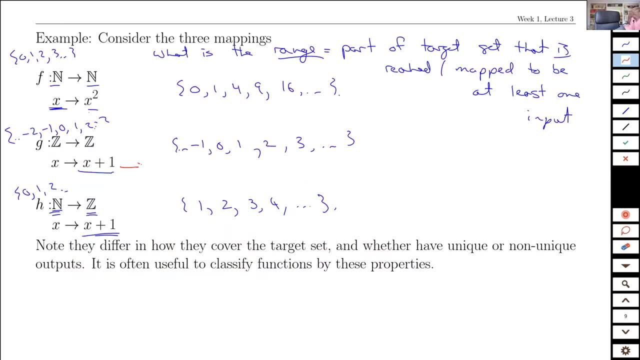 that is the input for that output, And that's true for no matter what value you pick on the other side. So, going back a slide here, this function here we would call surjective Okay, Because the entire collection of output values we can get is all of the integers that can. 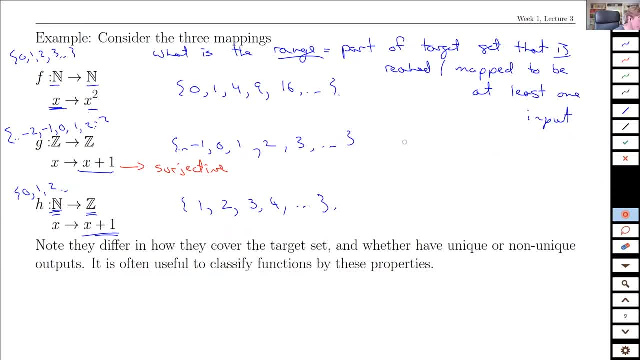 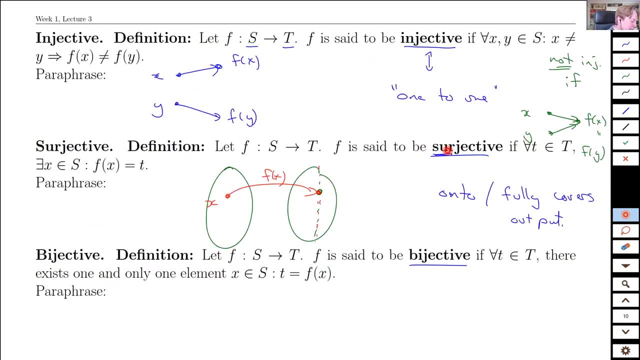 always find a way. If I pick any random integer, like 10, I can always find an input that would get me there. Here would be nine, Yeah, So we're looking at every. sorry, let me double check here. It's very similar to the vertical horizontal line tests. 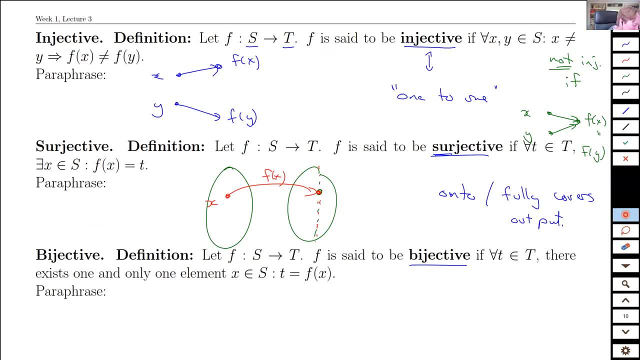 I'd have to think about that for a second or two to make sure I'm not springing up on you. But yes, it's got that kind of vibe. Sorry Being a function, sorry, let me just draw this quickly for a second. 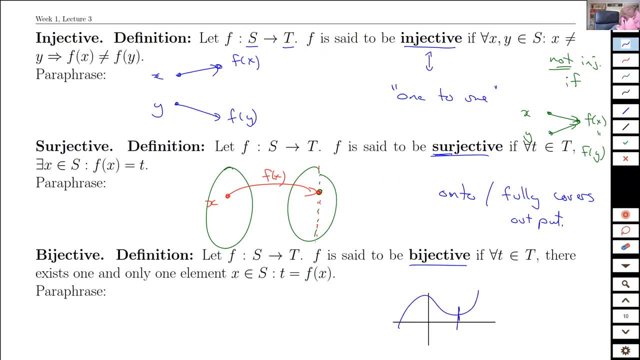 Being a function at all is the vertical line test, So we've already passed that. Bijective is actually the horizontal line test. it's both of those guys together. We never really talk so much in calculus about surjective. we never really care about covering. 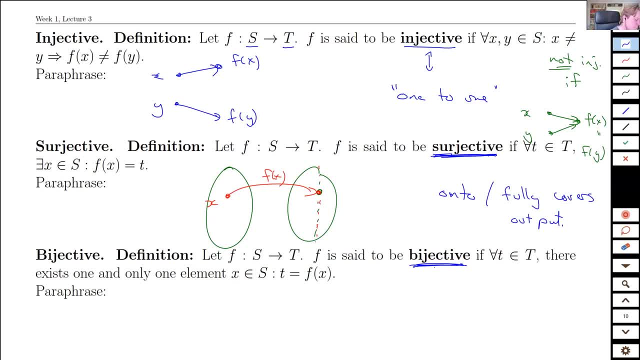 all the reals. That's not really a thing. Bijective is the combo Of injective plus surjective And this is invertible in a more stringent sense than what you're thinking about with the horizontal line test. And because this guarantees guarantees- I can't say guarantees invertibility- 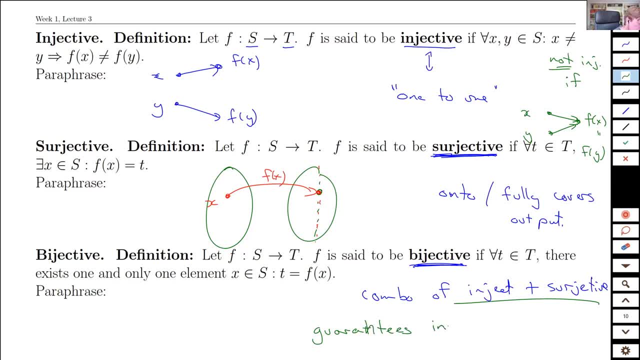 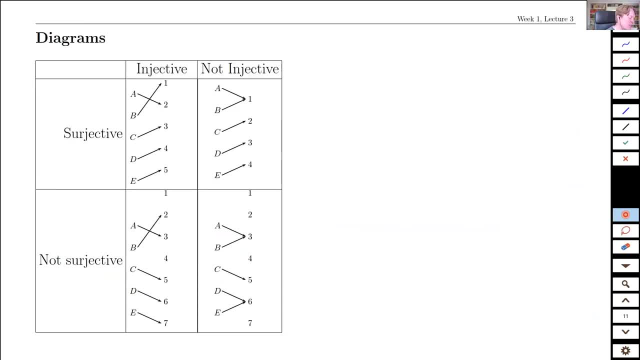 That would be possible if I just had surjective. Honestly, I find the diagram on the next page is the most helpful for this. So this is the both block here. Yeah, Yeah, Yeah, not categories, either one row or one column off. This not injective has two inputs that. 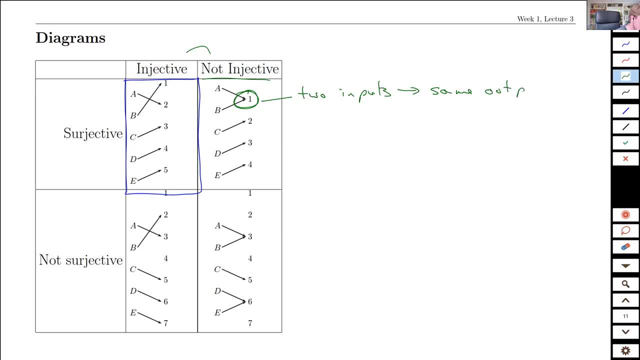 lead to the same output. That's not injective. When we talk about not surjective, that's where we have some lonely elements left over. Let me get rid of that. Lonely uncovered output values Again, if I look for surjective everything in this thing here, if you look down the column- 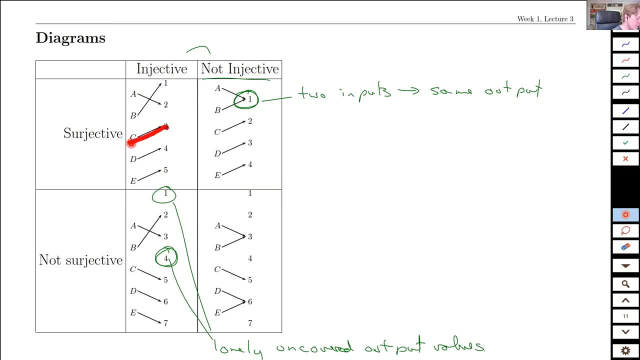 of outputs. can I get to one: Yes. Can I get to two: Yes. Can I get to three: Yes. Four or five: Yes. Over here same thing. Can I get to one: Yes, But not surjective. 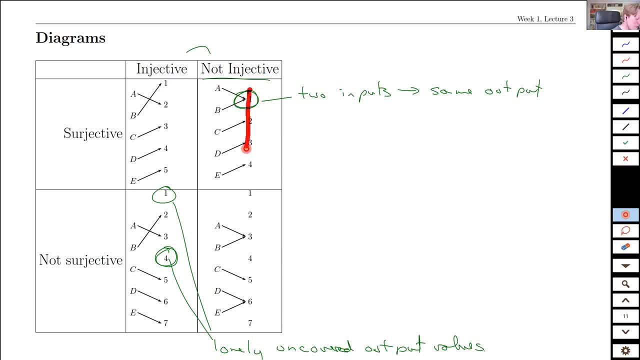 More than one way. So that's true. I'm covering all the outputs. Every output has an input, But it's not injective, because, well, I get to this one output from two different inputs. Then you can have the opposite kind of scenario. here Everything was covered, here Everything's. 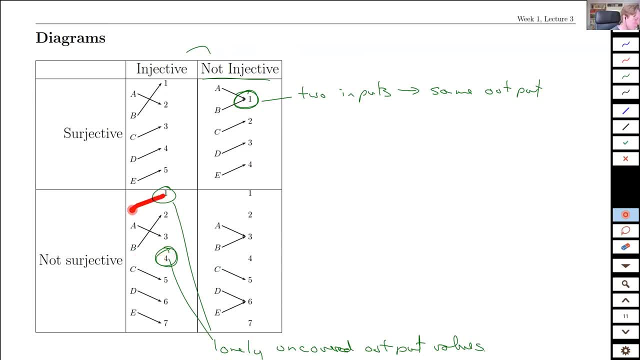 not covered here. The four doesn't have an antecedent in the function, The one doesn't. But for every value I do have I can go backwards. If there is a value here I get to there's a surjective. Sorry, it's injective, But it's not surjective because not every output. 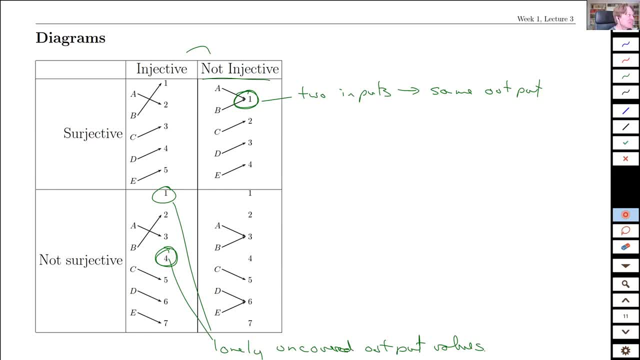 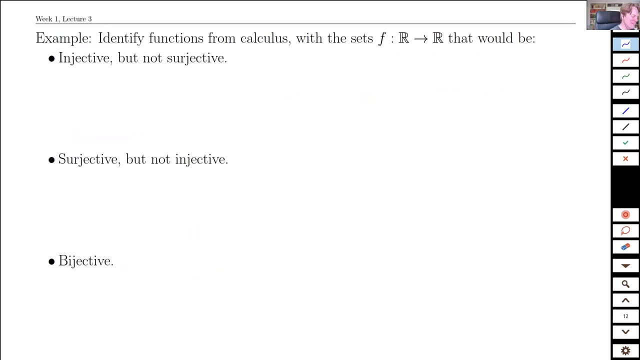 has a is found with this transformation. There's some values where the inputs don't map to a certain output value. Hoo-wee, All right. So again, let's put this in context for real-to-real functions. So maybe we can talk about the horizontal and vertical line. 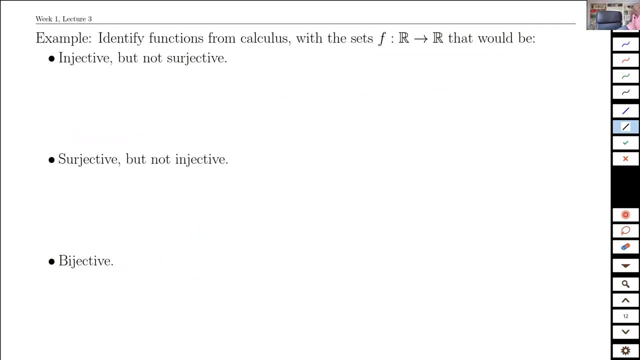 tests and things like that. So injective- injective, which again is not surjective, And it's sometimes helpful to think about those other expressions. Injective was one-to-one So, and I find that a little deceptive because that sounds like it's also invertible. It's 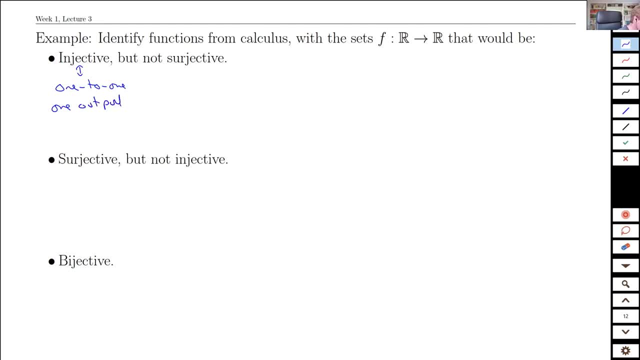 not One output equals one single input. That's really, I think, better capturing what we want here. So, if you think of a function that does that but is not surjective, there's actually a whole pile of functions that do this. 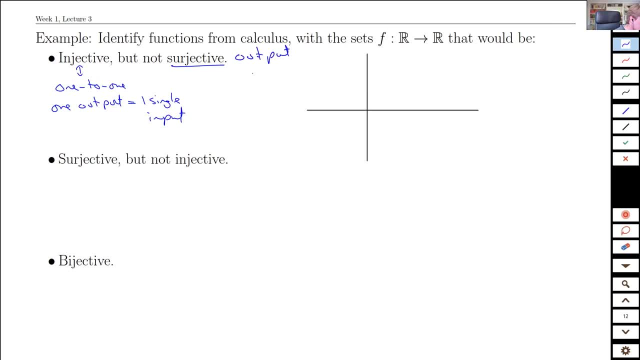 So surjective means the output is not all of the real numbers And so sorry, I don't have examples of mine here, I'm just going to blank. Oh yeah, yeah, Oh yeah. E to the x, of course. So Y equals E to the x. That graph looks like this: I know that every Y-value 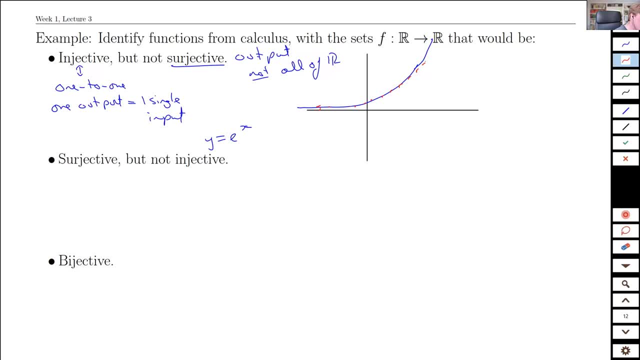 I pick. every Y-value I pick has this belief And, based on the Boolean, if this is positive, I benefit. I would get higher y sales cost. I don't care about fundamental market price pick. I can go back to a single x value and so it is injective but it's not surjective. 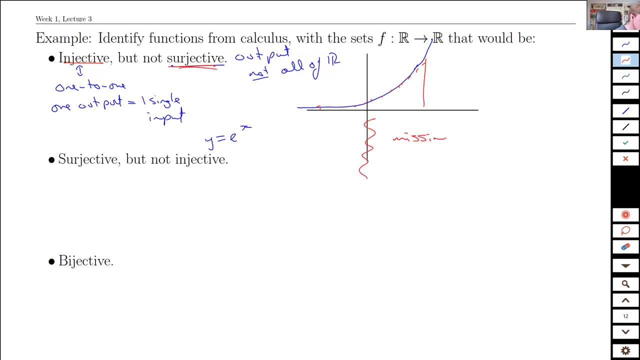 because I'm missing the zero and negative real outputs. Another function in that same vein would be something like arctan, just to give you another context. Arctan would have that same structure where I can certainly invert it, in the sense that if you give me a y value, any of the y values that are in there, I can go back to a single. 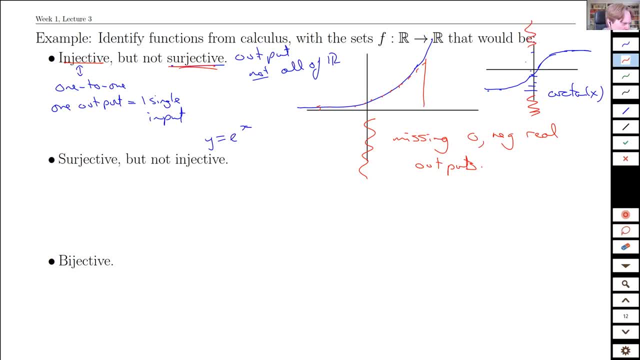 x value, but I'm missing part of the output domain. Now, bijective is almost easier than the one in between, so I'm going to do that first. So someone mentioned y equals x cubed. absolutely, that's a classic example of a bijective function. 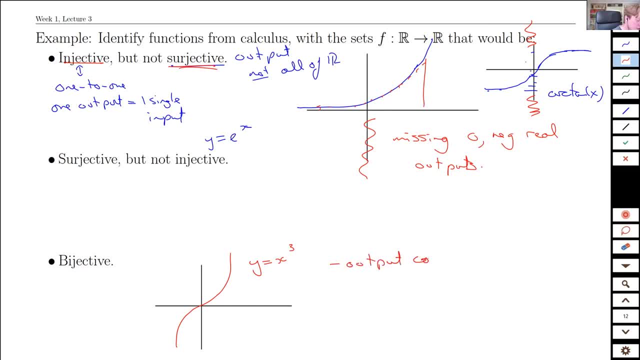 The output covers all the reals. in other words, this y value range here is infinitely large. I can get any y value that I want from some input and every y value I have is a single x value that gave rise to it. 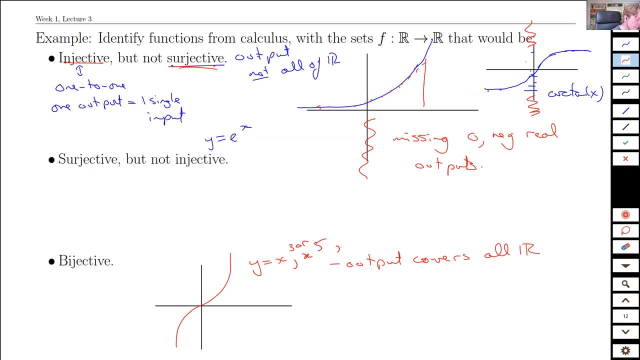 And so of course, everything in that family too, like x to the 5 or x to the 7, those are all perfectly bijective. One that's in the middle, it's actually kind of close to this. We can break it down. 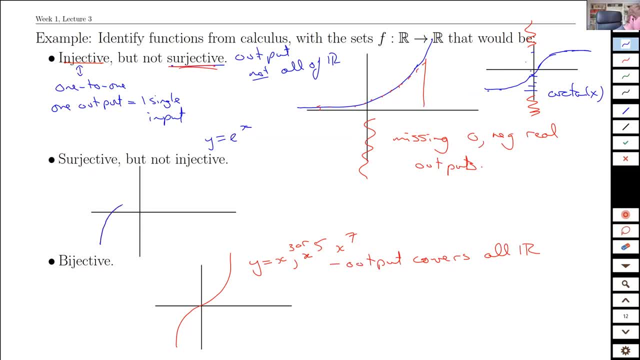 We can break the injective part by just having it loop back on itself. So I think this is x. yeah, let's just do the roots x minus 1, x plus 1.. This one, here we cover all the output range. eventually, this is a cubic and it's going. 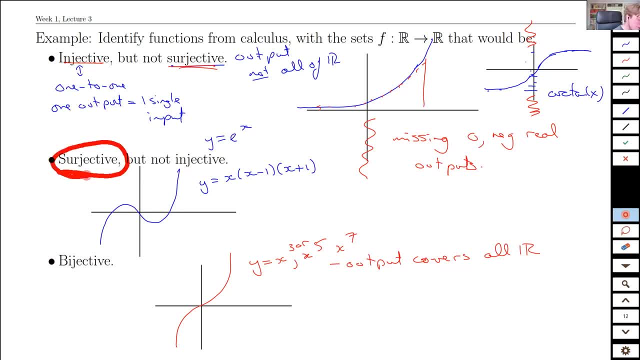 to go off to infinity and down to negative infinity. So cover all the output that's surjective output. cover all of r, But it's not injective. why? because if I have these two, let's take this y value here. 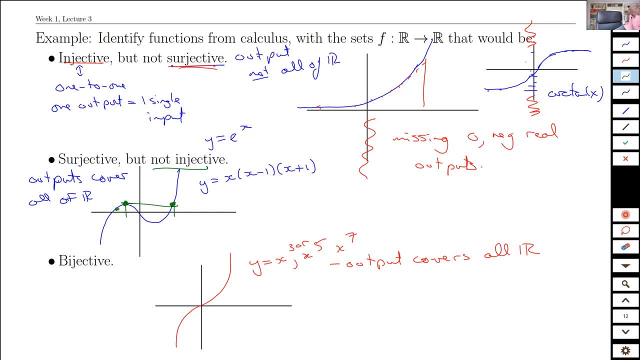 this y value here and this y value here, I can get the same y value, not every y value, but I can get the same y for those cases there with two different x's, And so that is obviously the thing that surjective is all about. 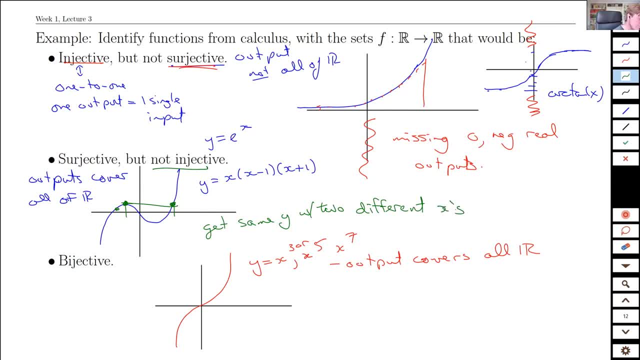 I'm sorry, injective It's the same y with two different x's. Yeah, and you can actually feel this, right, This fails the horizontal line test, so it's not invertible. So not injective means not invertible. 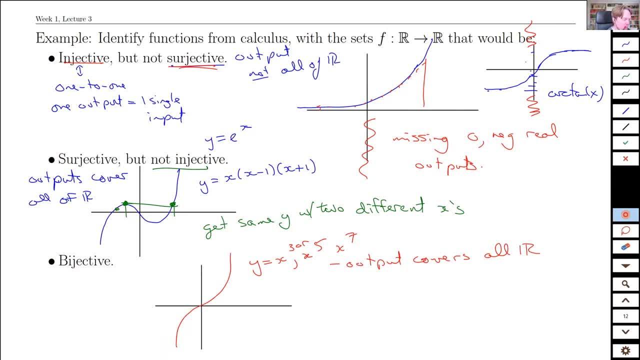 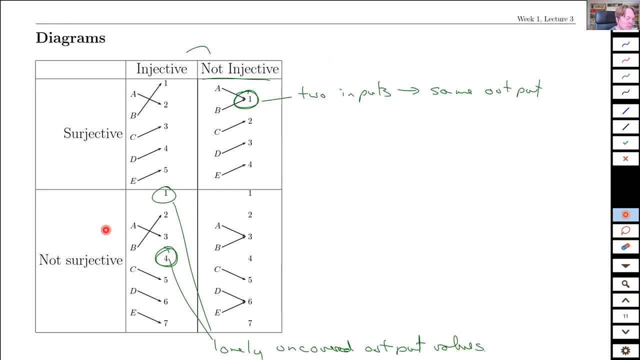 Whereas this one here is glorious, it's bijective, it is invertible, has all those nice properties. So you're going to have to have these kinds of definitions or properties of functions pretty well understood in being able to translate the new terminology. 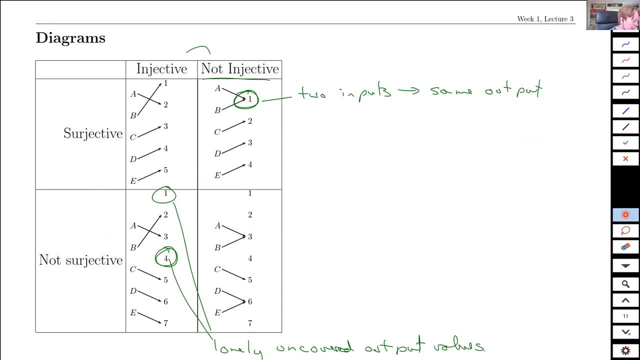 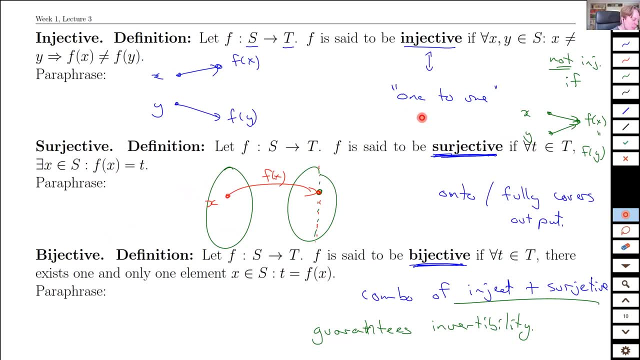 If you haven't seen it before: injective and surjective into something that means something to you. If you find the one-to-one and onto helpful, then by all means use that. As I mentioned in web work, we're actually going to use these phrases. 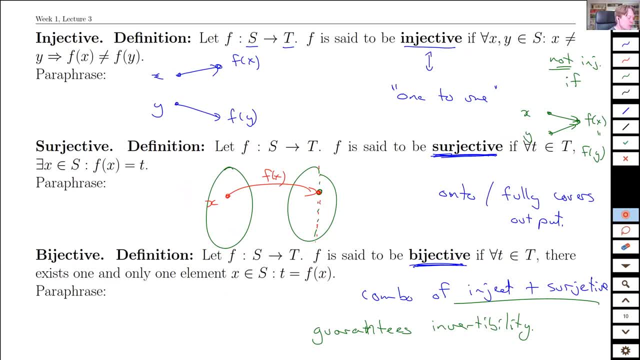 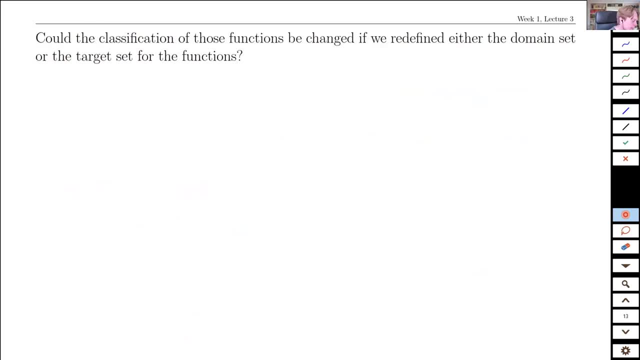 I think it's in the sixth question in the web work, So be prepared for those kinds of questions and to using that kind of terminology, This question here. I'm just trying to point at the importance Of the domain set or the target set. 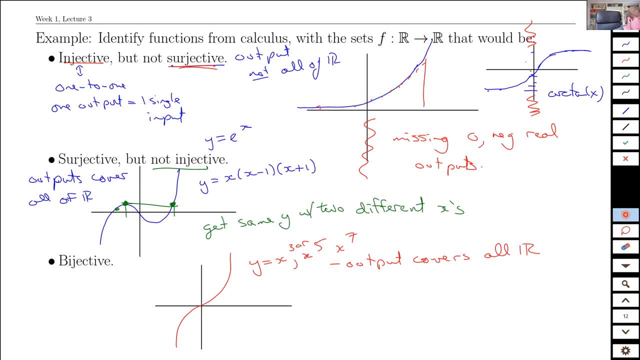 If we take a look at e to the x, like, e to the x is a great function. It's definitely injective. It's one-to-one in the sense that every y value just comes from one x. The only reason it's not surjective is because we are missing the negatives and the zero. 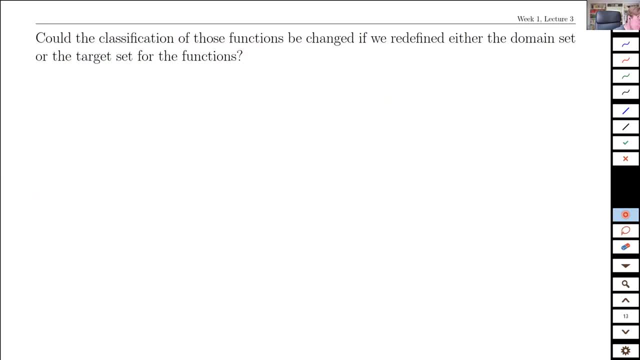 value. Those are not possible outputs for the exponential function. So we could fix that by just choosing a different function. So we could say: let g be a function that maps x to e to the x, And we're going to map the reals in. 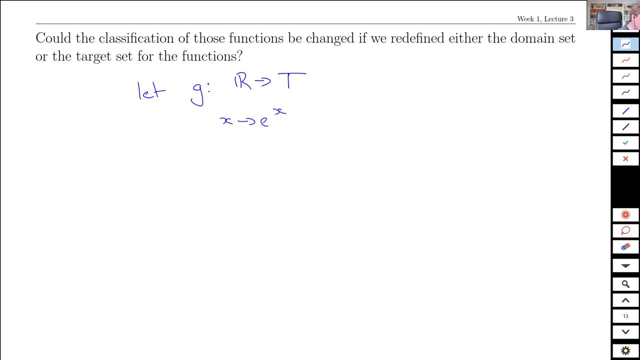 That's fine. And we're going to map to some set called t, where t is all the values x that are reals, but that the x's are greater than zero. And what does that do? Well, it basically says: oh, I'm only interested in output values that are I shouldn't include. 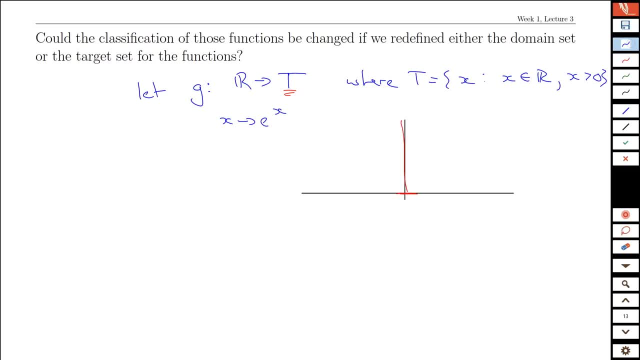 the axis here, but zero and above zero here, In which case the exponential function y equals e to the x, Does in fact cover every single value in t. Output of e to the x is all of t, So g is surjective here. 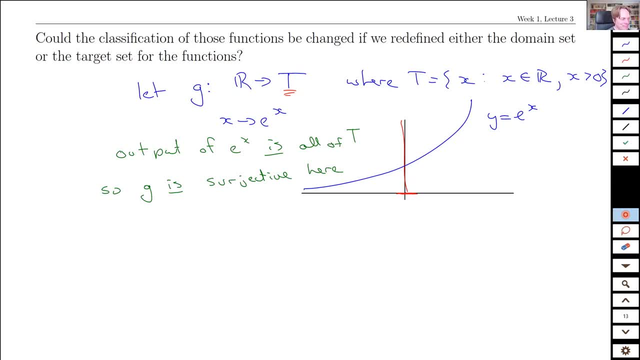 So we can sometimes tweak our sets so that we get a property that we want, And this very much is like the arc sign. We can do that in a lot of our shenanigans where we had we were trying to invert a function. 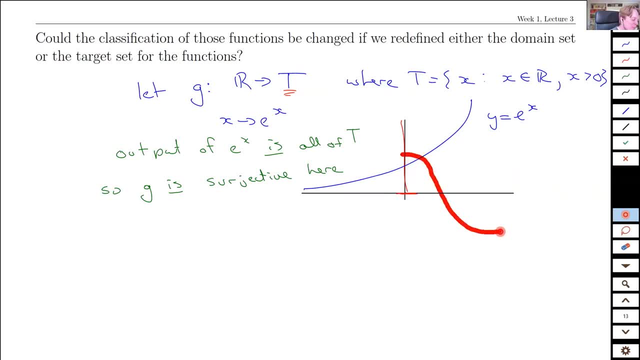 that went up and down a bunch of times. We said, well, let's not do that, Let's pretend we're only looking at some part of the interval and we limited our domain. So this is a fix you've seen before. Yeah.